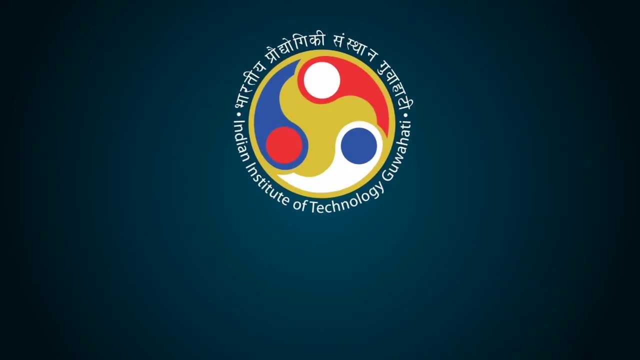 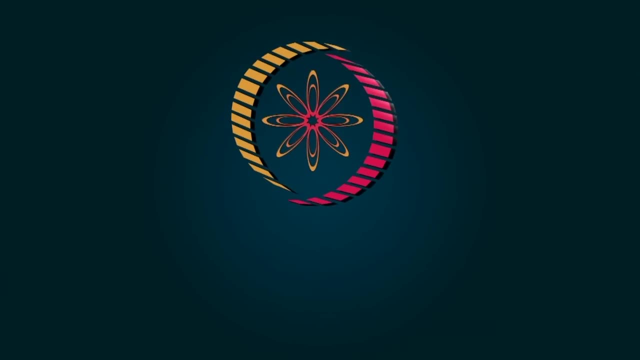 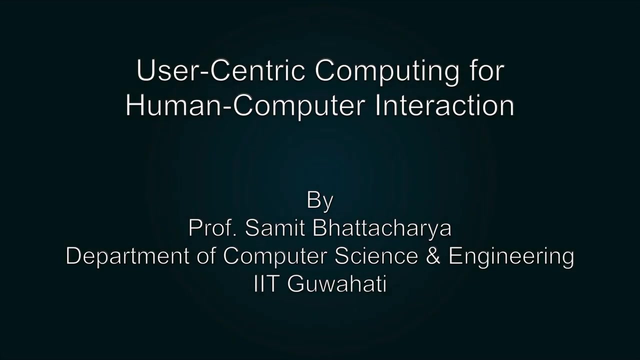 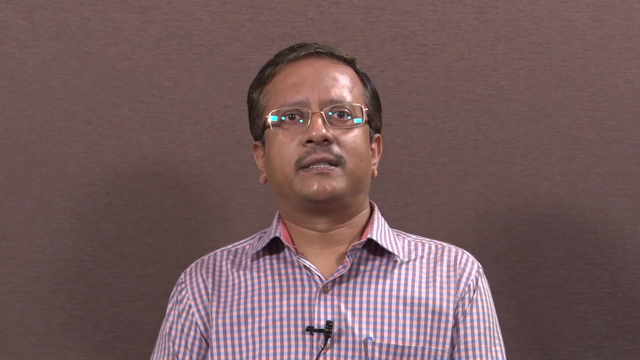 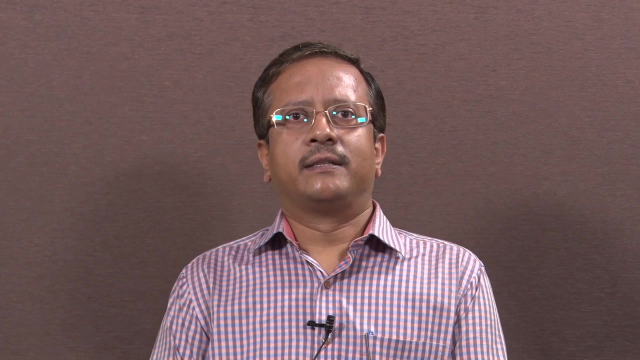 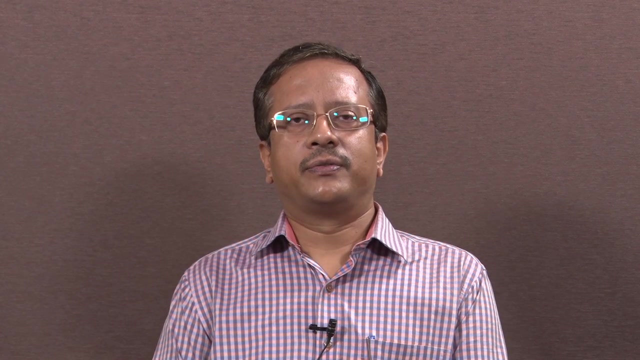 Thank you for watching. Hello and welcome to lecture number 29 in the course User-Centric Computing for Human Computer Interaction. So in the previous 28 lectures we have learned about many concepts related to this course. So if we quickly have a recollection of what we have learned, 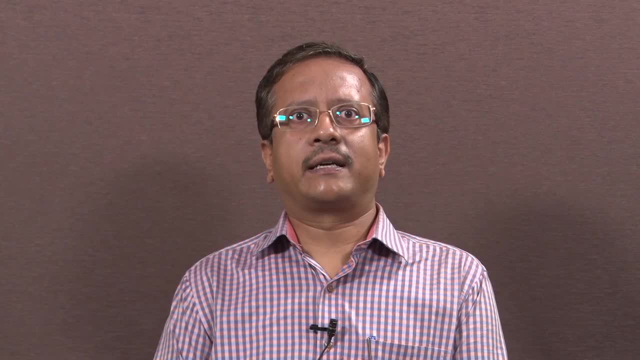 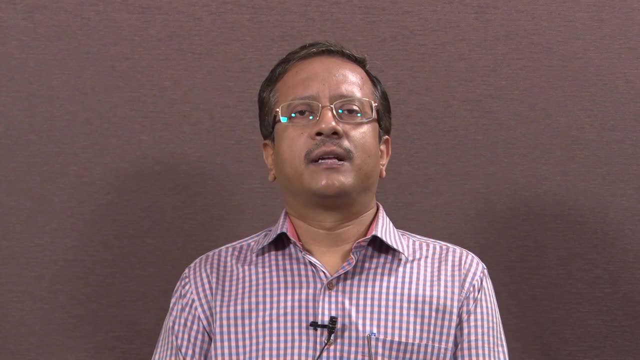 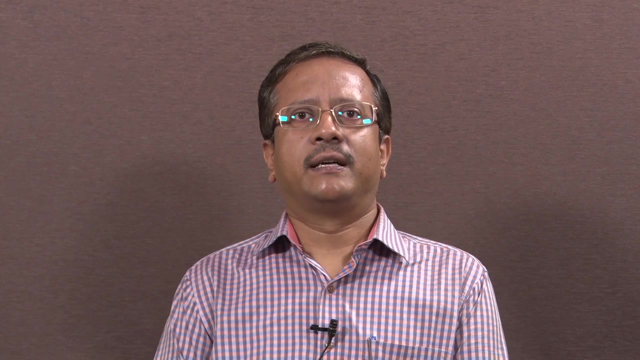 So we started with a discussion. So we started with a discussion on overall interactive system design process. what are the stages involved? Then we discussed about the importance of computation in the design of interactive systems and we have discussed one computational framework In the subsequent 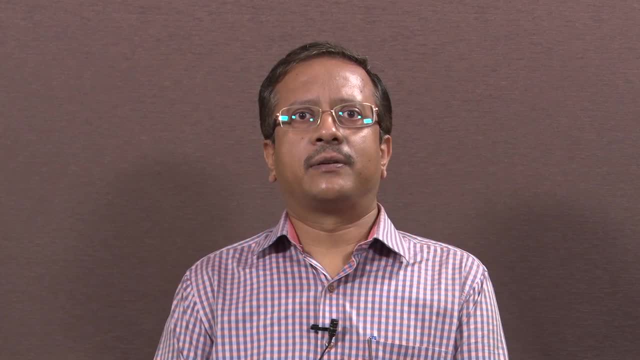 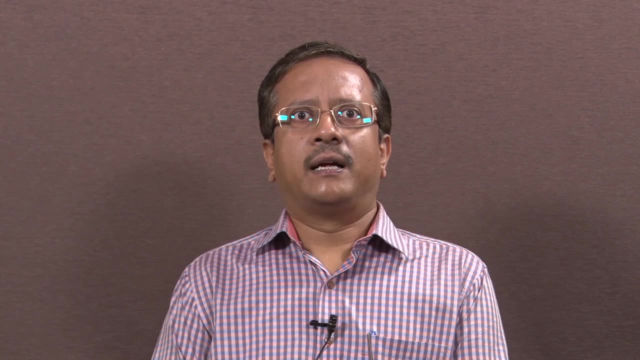 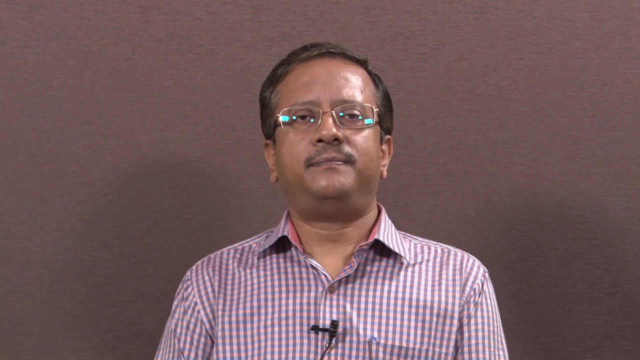 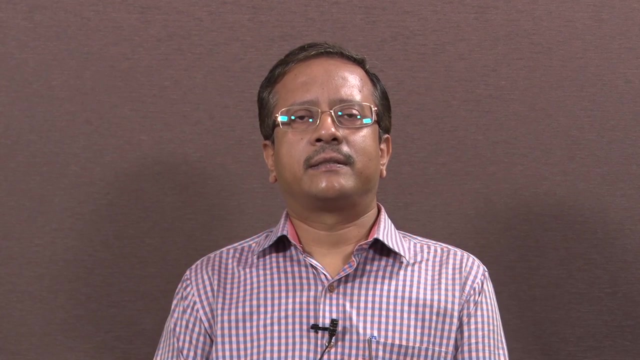 lectures. we discussed about user models, particularly computational user models, which is a very important component of the framework. We have also discussed in details about the empirical research method. So one more important concept remains to be discussed, which we are going to discuss starting from today, that is, how to evaluate interactive systems. 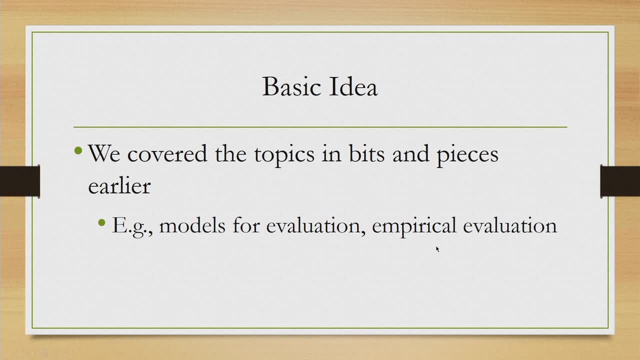 So when we talk of evaluation, if you recollect the previous lectures, we talked of this concept: a few classes available. 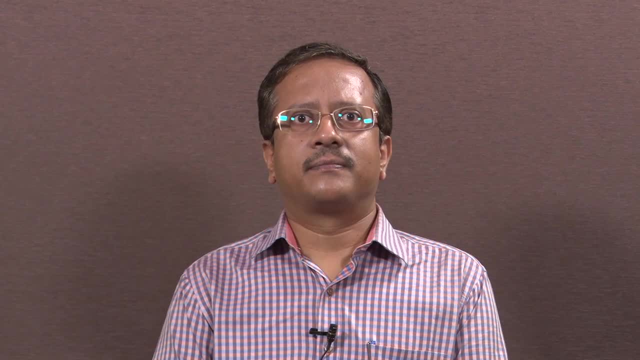 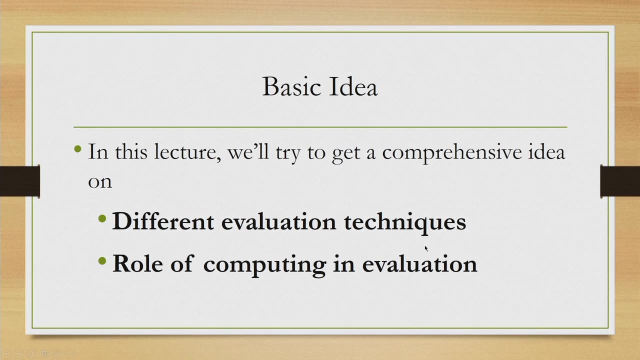 and pieces earlier as well, when we talked of the use of models for evaluation or in the context of empirical studies. Now, in this lecture, we will try to go a little deeper. We will try to have a comprehensive understanding of the concept of evaluation in the context. 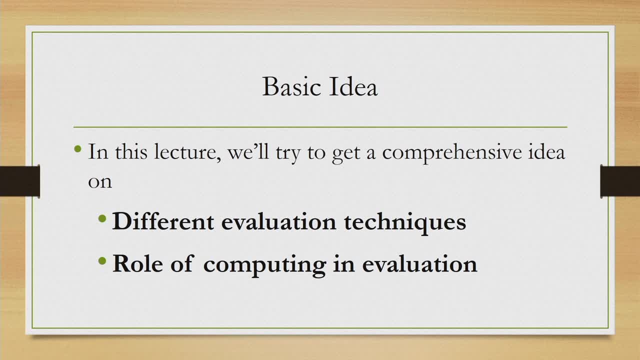 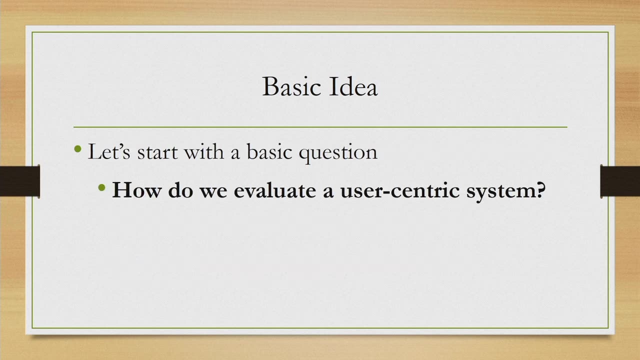 of user centric design, and we will try to also discuss what role computing plays in evaluation of user centric systems. So, in order to start, we will start with a very basic question: How do we evaluate a user centric system? So, if I ask you this question, 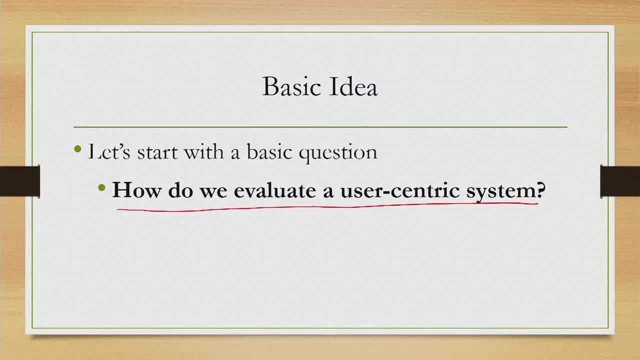 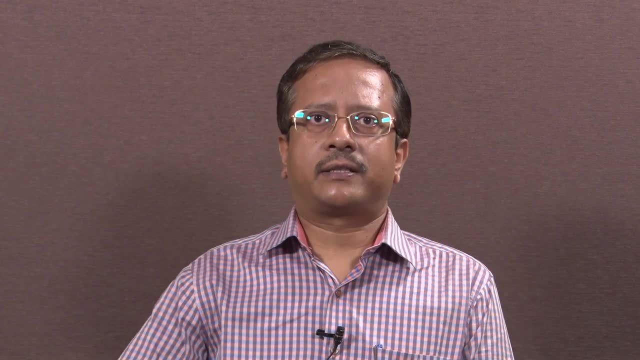 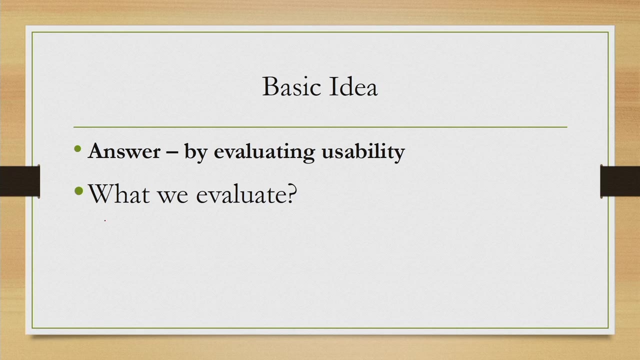 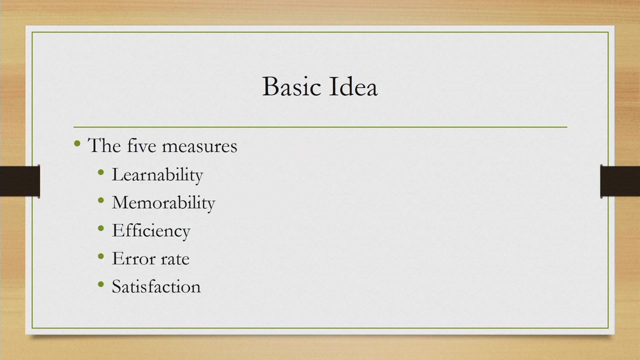 What will be your answer? The most straightforward answer is, of course, by evaluating usability of the system. but the next question is what we evaluate when we talk of evaluating usability. What are the things that we evaluate in usability? Now, in one of the earlier lectures, if you may recollect, we mentioned five things. 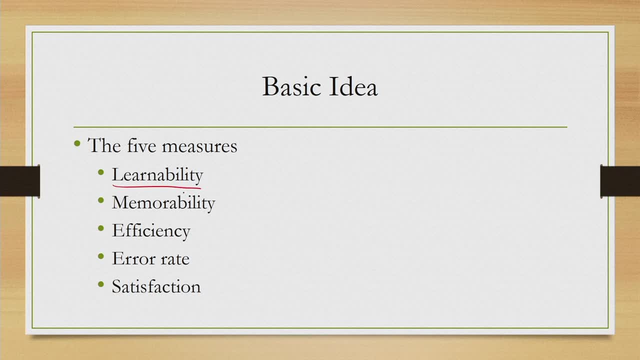 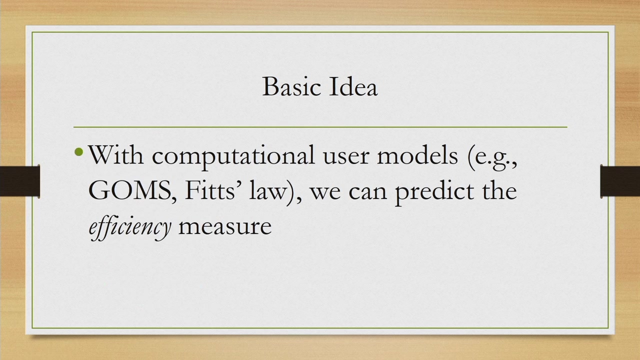 Five measures of usability. Those are learnability, memorability, efficiency, error rate and user satisfaction. So when we say that we want to evaluate a system in terms of usability, what we indirectly refers to is to measure these components of usability, The computational models that we have discussed. 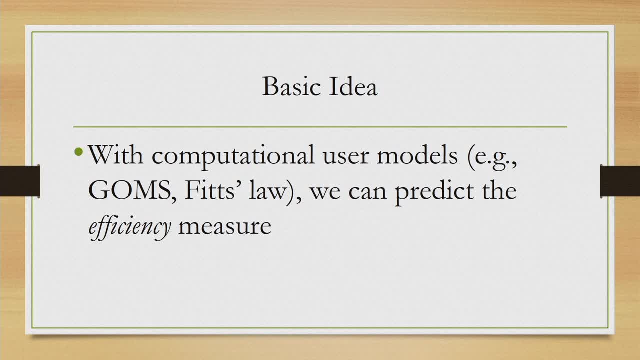 earlier Can be used for the purpose, as we have seen during the discussion on those models. Models such as GOMS or the Fitts law or the Hick Hyman law can be used to predict performance measures that are related to the efficiency measure of usability. 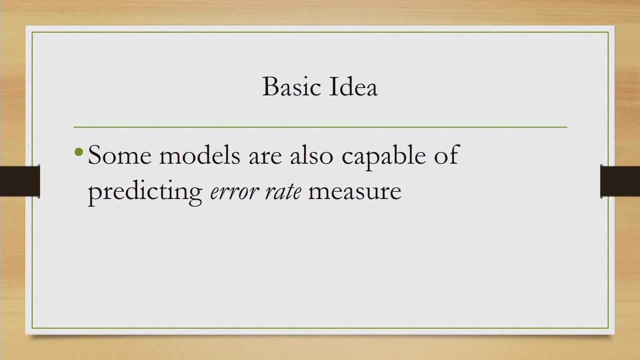 Some models are also there which can be used to measure error rate. So these are the models that we have discussed earlier. Now let us talk about performance measures. Performance measures- Performance measures- can be used to measure error rate. However, the formal models that we have discussed can also be used to measure certain quantities. 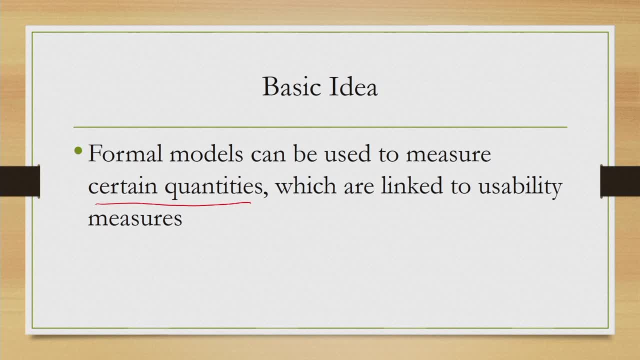 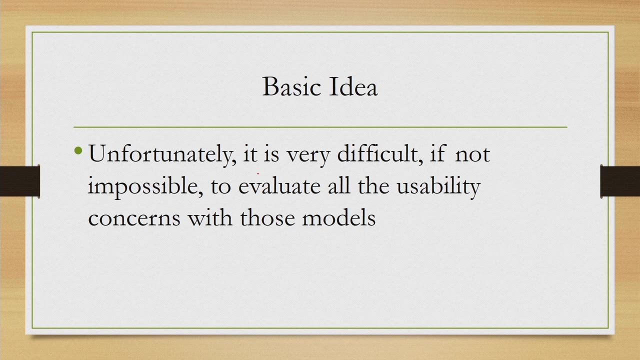 which can indirectly be linked to the usability measures. These, again, we have seen during the discussion on the use of formal models. But the point is that it is very difficult or may be impossible. It is very difficult, It is very difficult, It is very difficult. 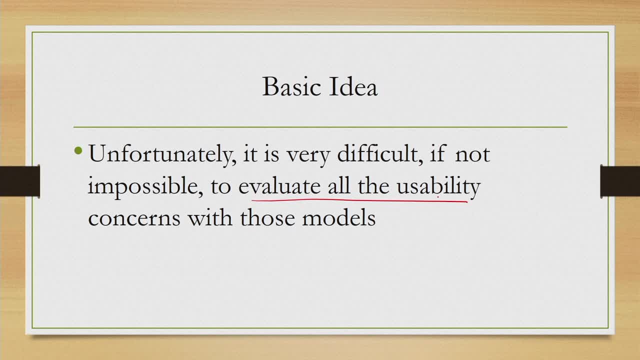 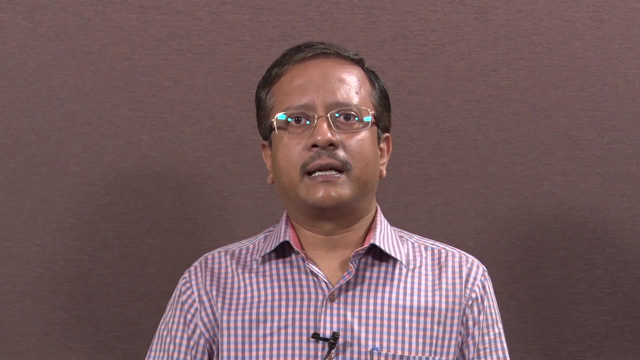 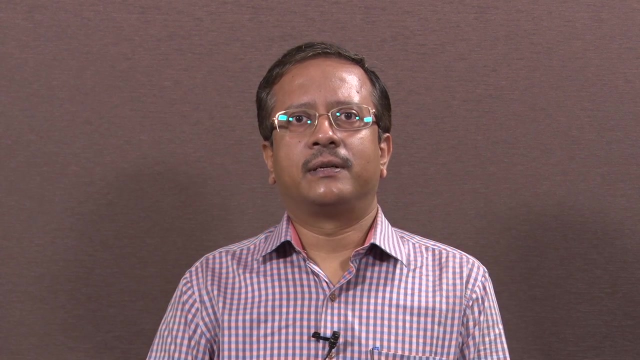 It is very impossible to evaluate all the usability concerns with these models. So the models can be utilized to measure few things, such as efficiency, error rate. but there are certain components of usability which may not be possible to be measured with these formal models. 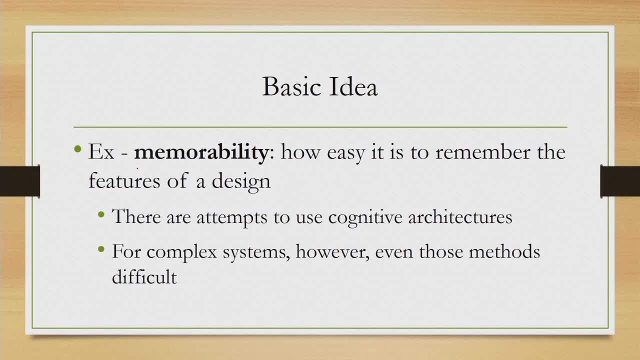 For example, For example. For example, If we saidрип assuranceвод is possible, people use oper flexibility. how can that be measured with formal model? So what is memorabil�? It essentially refers to the ease with which we can remember the features of a design. 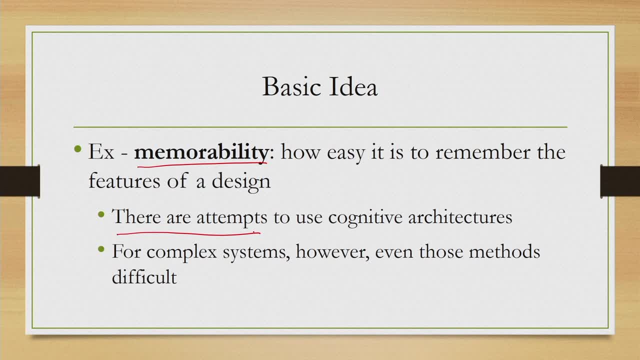 That is the definition, which is, of course, somewhat vague- cannot be quantified easily, And there lies the problem: how to measure it? Now, there have been attempts to measure. Unfortunately, the designers tend to guarantee that it will go well with their memory ability. 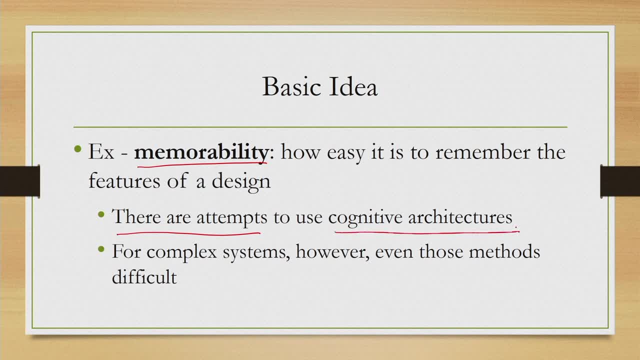 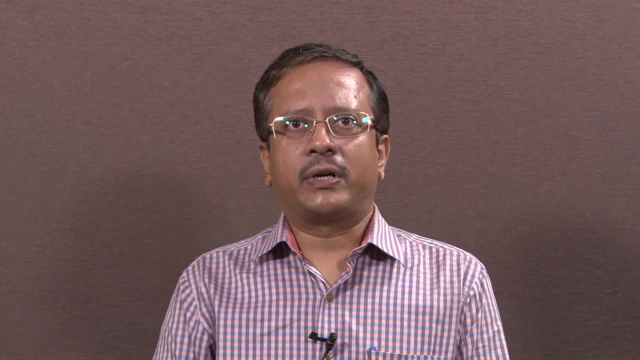 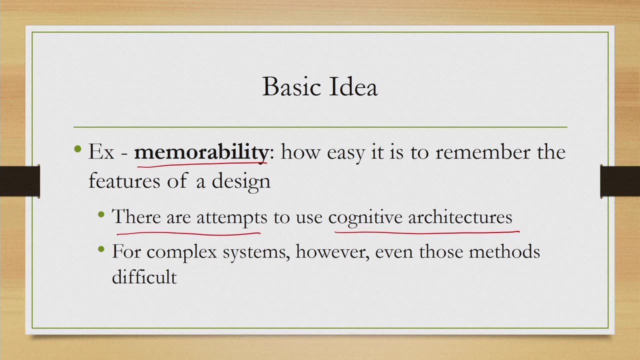 It has been a necessity There might be originate Now these cognitive architectures we have not discussed earlier. this is an advanced form of user models and they are quite complex. but even with cognitive architectures it is possible to measure memorability of very simple systems. 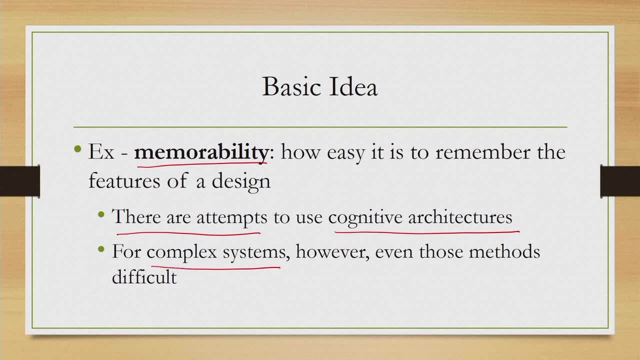 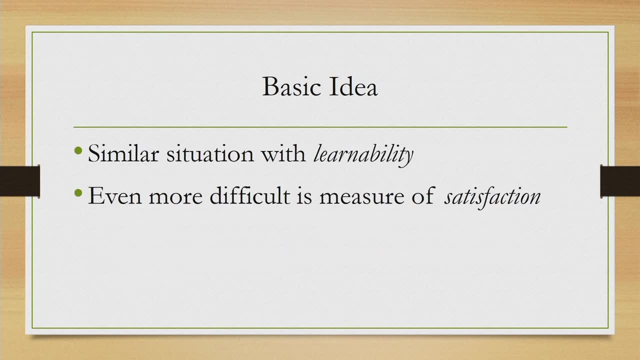 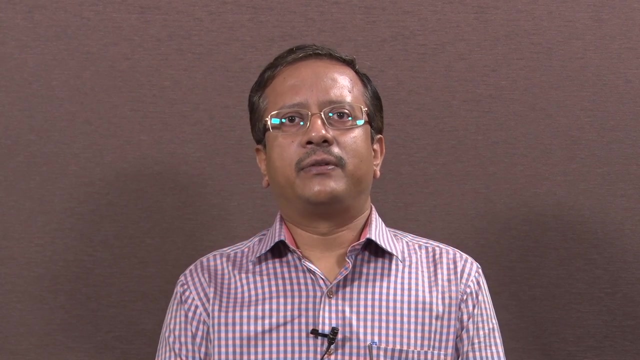 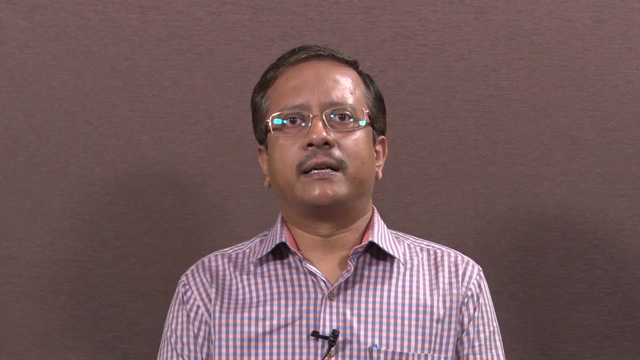 For complex systems, even such advanced techniques such as the cognitive architectures will fail. Similarly, there is an issue with measurement of learnability or satisfaction. So, in a nutshell, what we can say is that we can use models, whichever we have learned earlier, to measure, say, the error rate or the efficiency of the model. 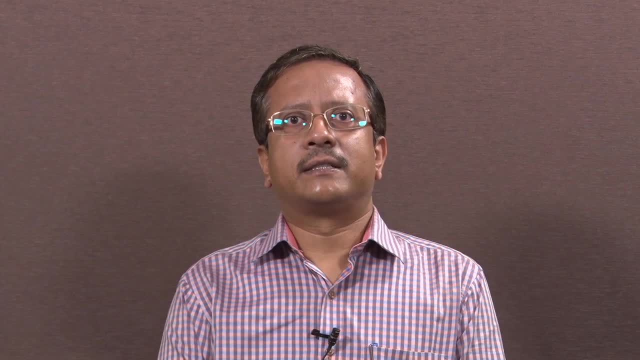 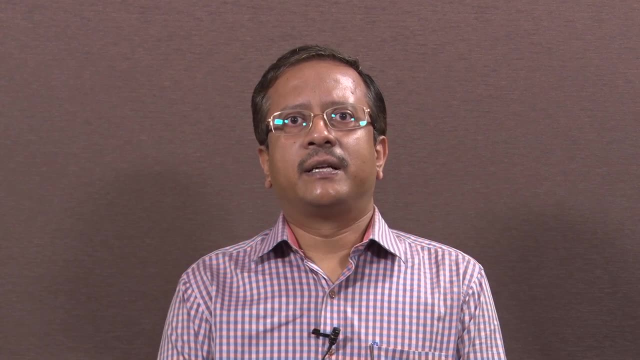 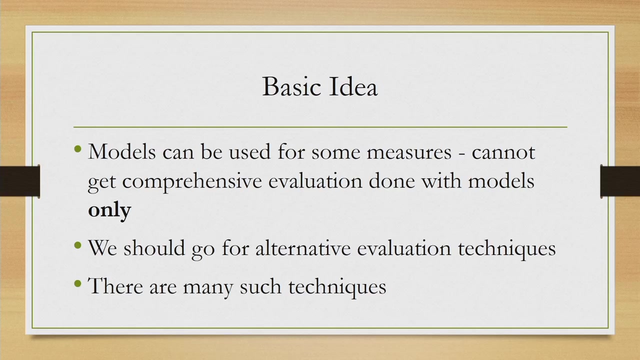 We can see, but these models may not be sufficient or suitable to measure memorability, learnability, subjective satisfaction. So some components of usability can be measured with models. some may not be measured with models only. So, then, what we need? 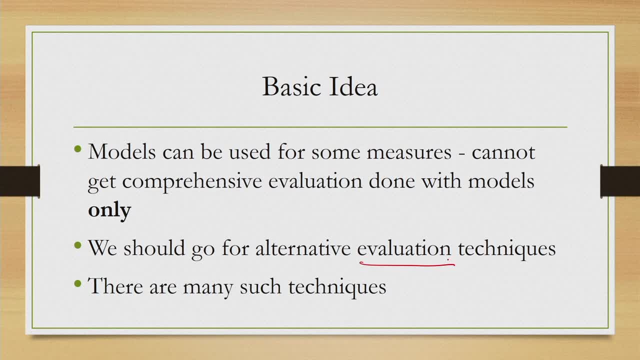 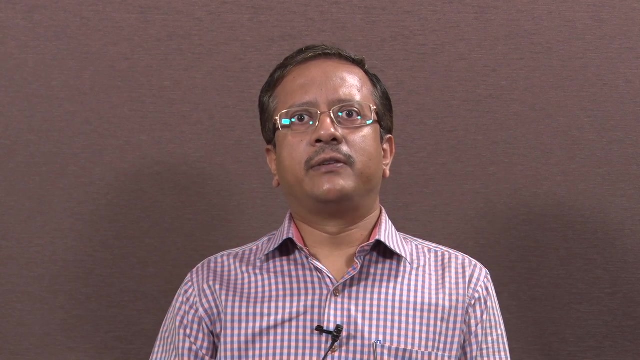 We have to go for alternative techniques to evaluate those systems. So, given a system only with models, we may be able to evaluate its efficiency or error rate, but we may not be able to evaluate memorability, learnability, satisfaction. So overall usability measurement or overall usability evaluation may not be possible. only 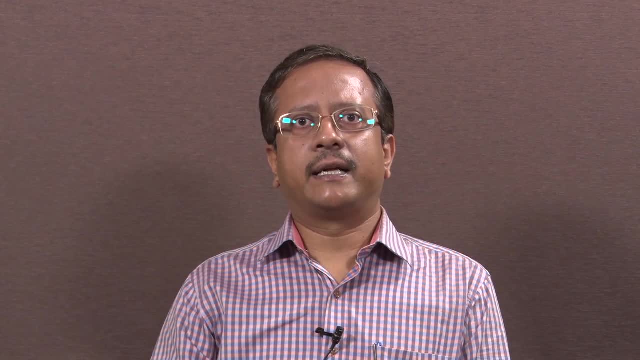 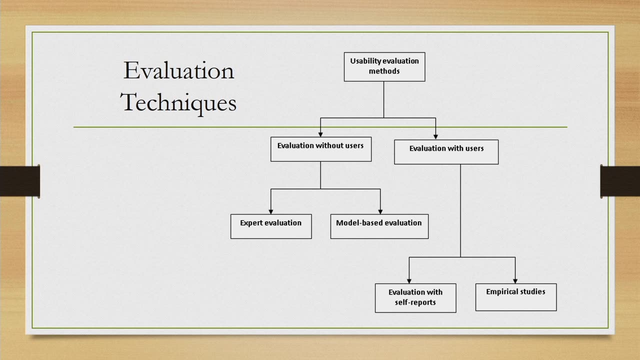 with models and we have to go for alternative evaluation techniques. There are, in fact, many such techniques available. We may categorize all these techniques in the form of a hierarchy, which is shown here. So all the evaluation methods may be divided into two broad categories: evaluation without. users and evaluation with users. 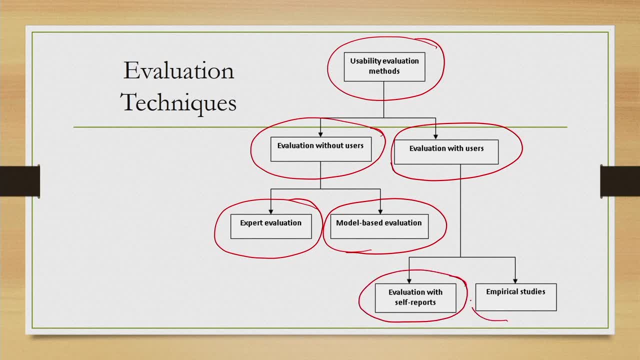 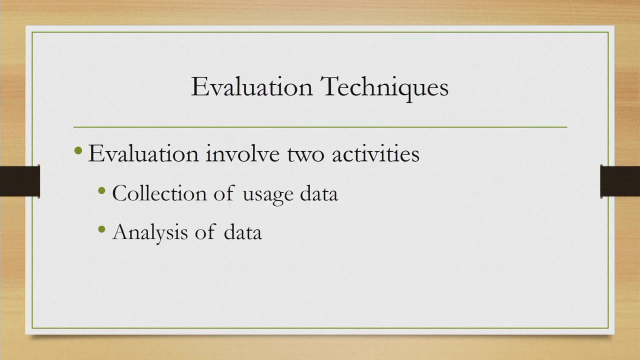 One is evaluation with self reports and other one is empirical studies, So broadly, all the evaluation methods we can categorize into this hierarchical form. There is another way to view this. Before we discuss that, let us try to look at another aspect of evaluation. that is, how. 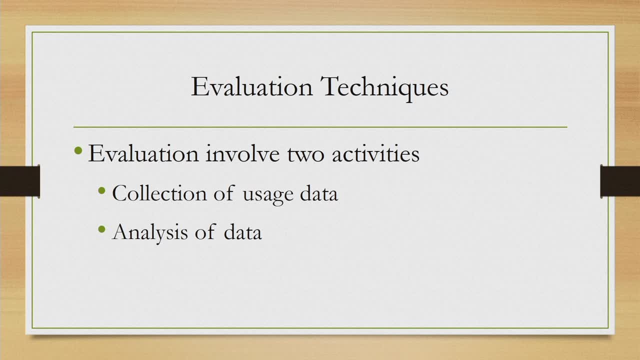 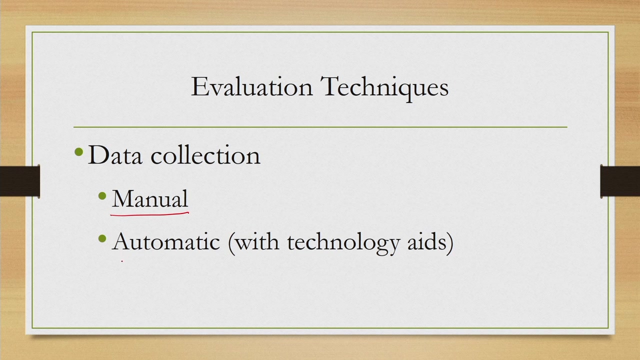 we perform the evaluation. It involves two stages or two activities. one is collection of data, other one is analysis of data. Now, if you may recollect, in a previous lecture we mentioned that the data collection can be performed either manually, through intervention of a human observer, and also it can be performed 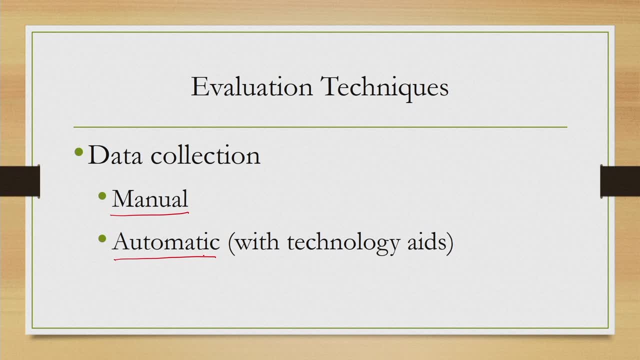 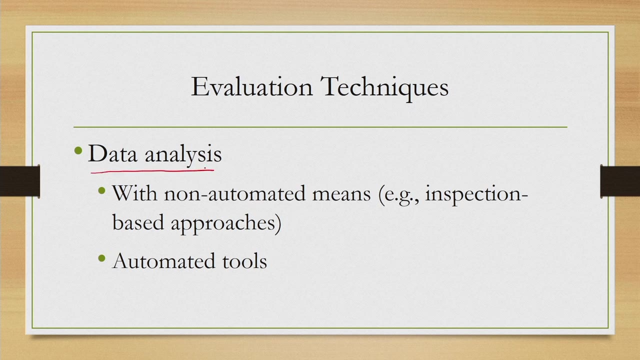 automatically with the use of technology aids such as computers, recorders, sensors, computers, etc. and so on. Similarly, analysis of data can also be performed in different ways. We can have non-automated means of analysis, For example inspection based approaches, or we can have tools to perform the analysis. 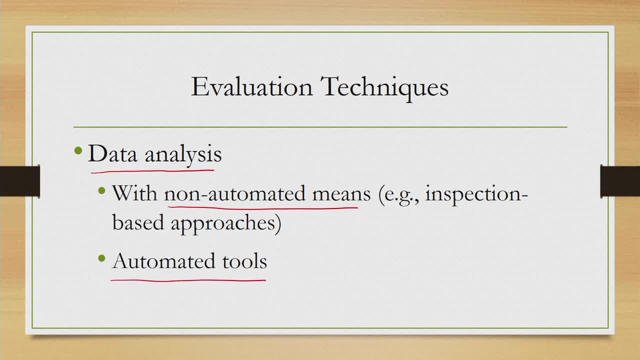 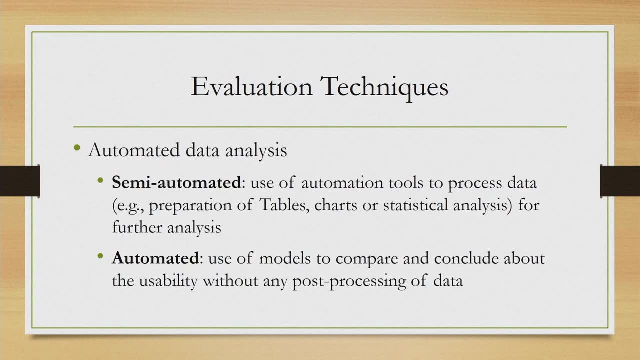 automatically. Now these automated Analysis, Analysis, analysis tools and the use of tools to perform data analysis automatically can again be divided into two subcategories. So automated data analysis can be done in either of the two ways. one is semi automated approach, other one is automated approach. 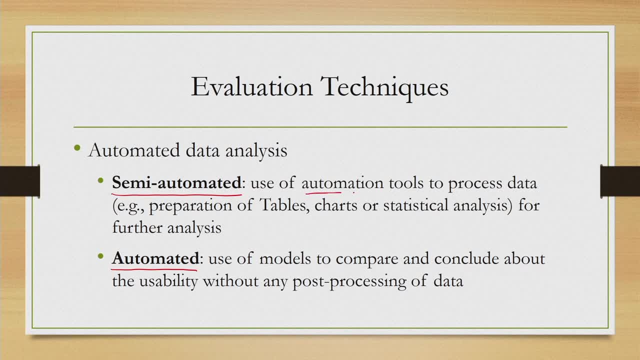 So in semi automated approach, we use automation tools for processing of data primarily- For example, preparation of tables, charts, statistical analysis- and these help us in further analysis of the data, which we need to do, sometimes manually, Ok. However, in case of purely automated data analysis approach, we use models to compare. 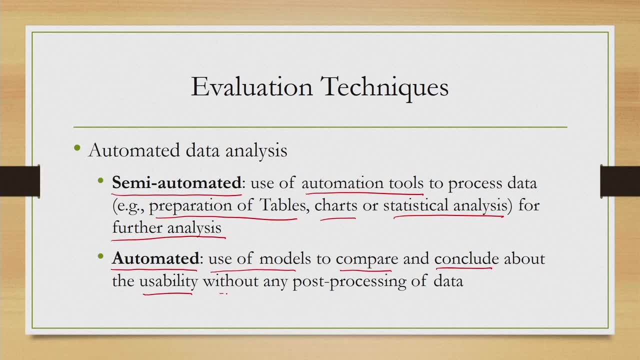 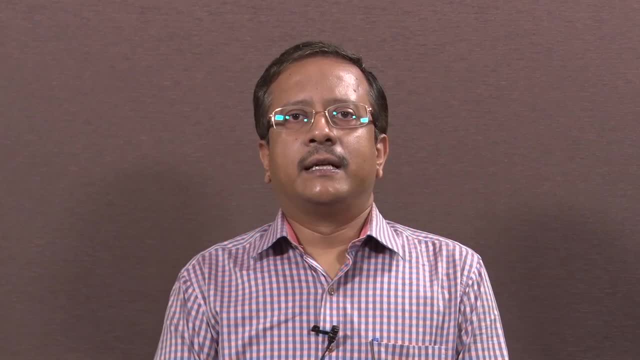 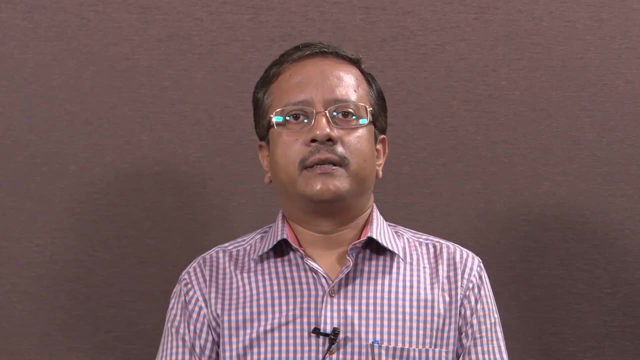 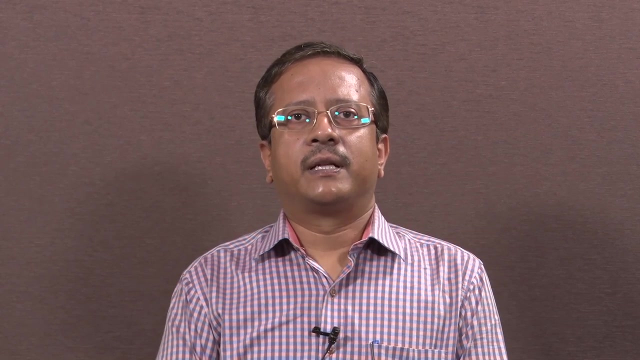 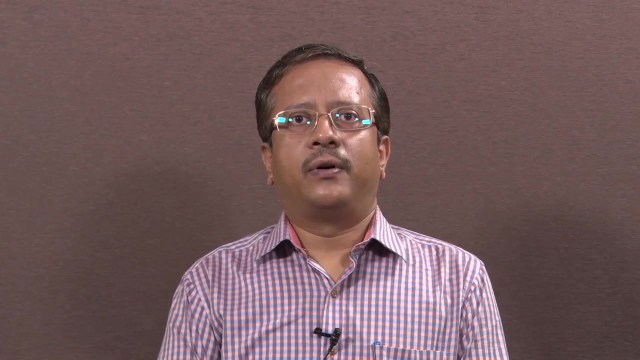 and conclude about the usability without any post processing of data. So to summarize, any evaluation involves two activities: data collection and data analysis. Data collection: we can do it either with manual intervention or manual intervention, Ok- With the use of automated tools. Data analysis, also, we can perform in a non automated way or in an automated way. 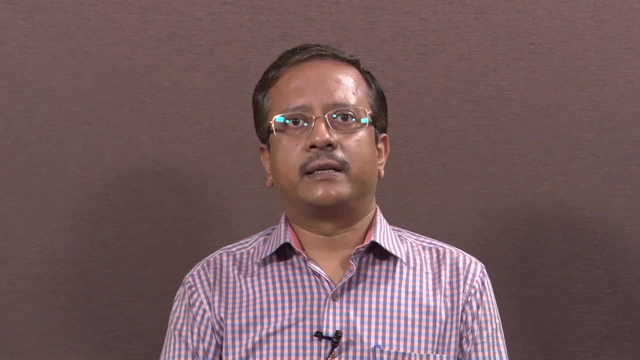 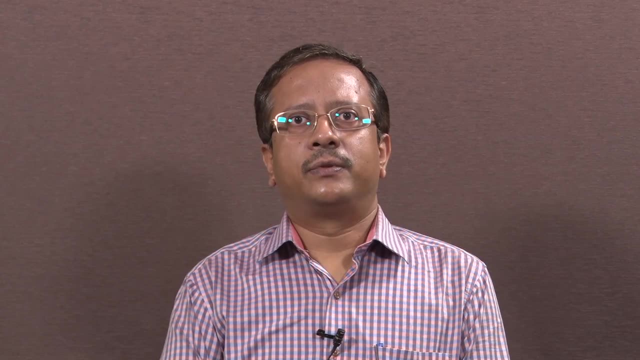 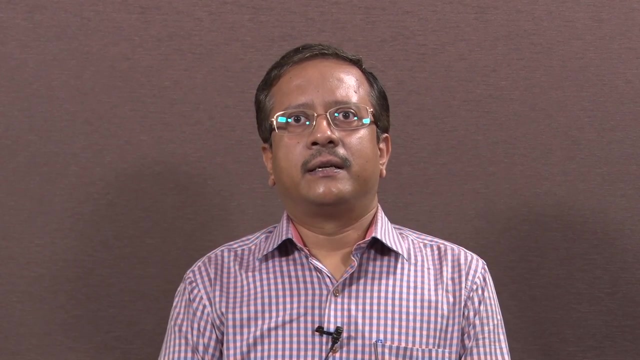 In automated data analysis approach, there are two categories. In one category, which is called semi automated analysis, we use tools- automation tools- to primarily process the data, rather than finalization- Ok Ok. And in fully automated approach, we use models to analyze and conclude about the data without. 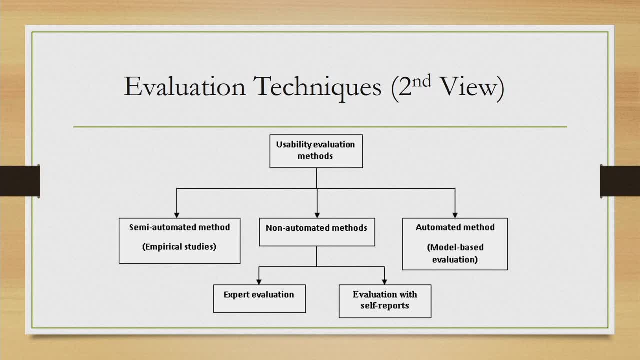 any post processing. So, based on the way we collect and analyze data, we can have a different hierarchy of usability evaluation methods than the one we have discussed earlier. In this hierarchy we have three broad categories. One is semi automated method, one is non automated method, one is automated method. 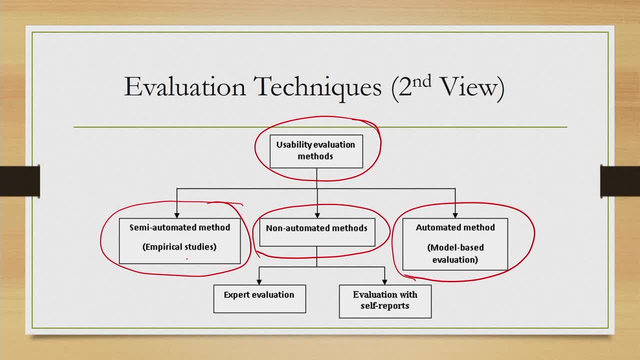 The empirical studies that we have discussed earlier comes under semi automated method, Now under non automated methods. there can be two categories of evaluation methods. One is expert evaluation And the other is non automated evaluation. The other one is evaluation with self reports, And under automated method we have the 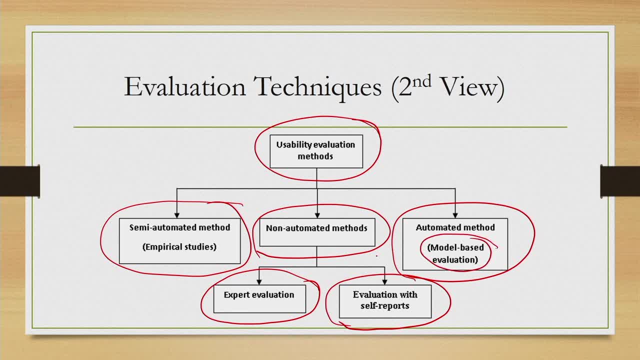 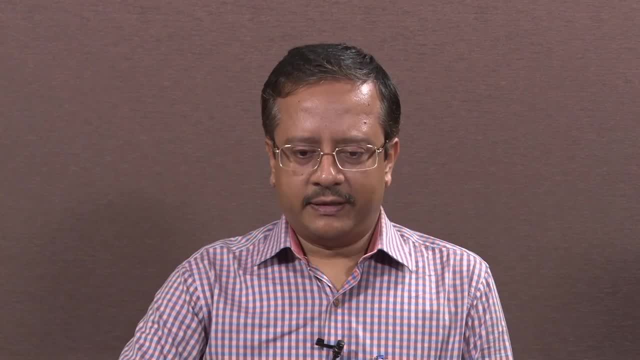 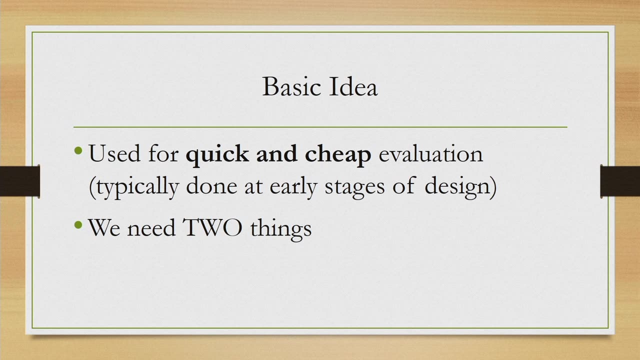 model based evaluation. Now let us try to understand these techniques one by one. So we will start with expert evaluation- What we mean by this. So when we are talking of expert evaluation, it is essentially referring to an evaluation method that is used for quick. 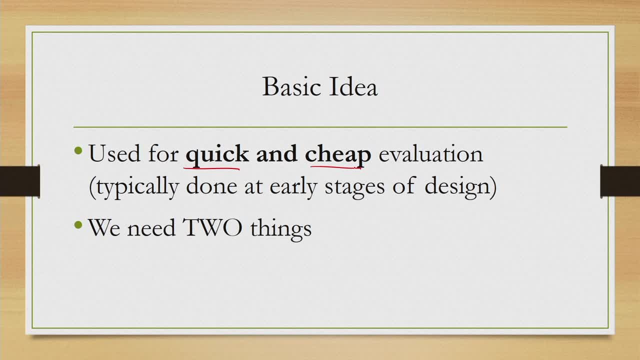 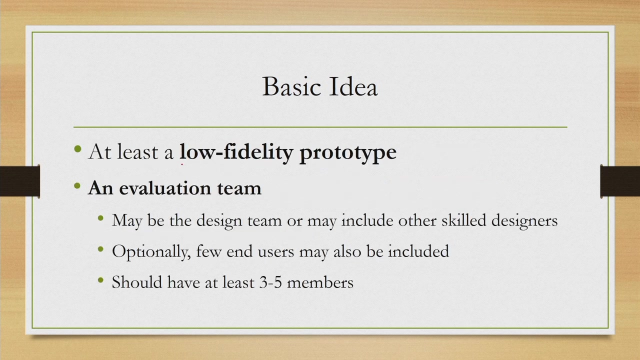 and cheap evaluation, and typically this is done at early stages of design, when lots of iteration takes place. In order to perform expert evaluation, we need two things. What are those two things? The first thing is a prototype, So we require at least a low fidelity protot可以减弱上限的游戏模型 En zdrab Buger method. we require at least low fidelity proto type. 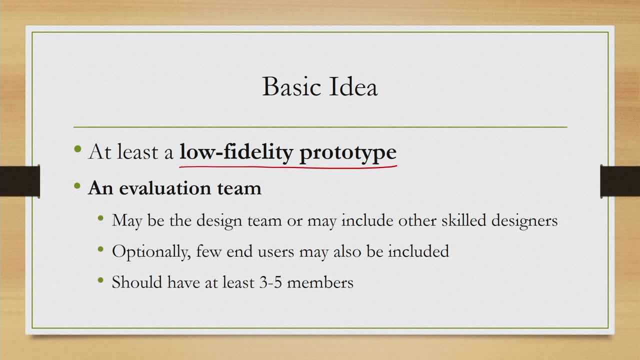 And the second thing that we need is an evaluation team, which should have at least three to five members. Now who are these members? They may be from the design team or may include some other skilled designers who are not part of the design of the particular product. optionally, we may also include few end users in the team. 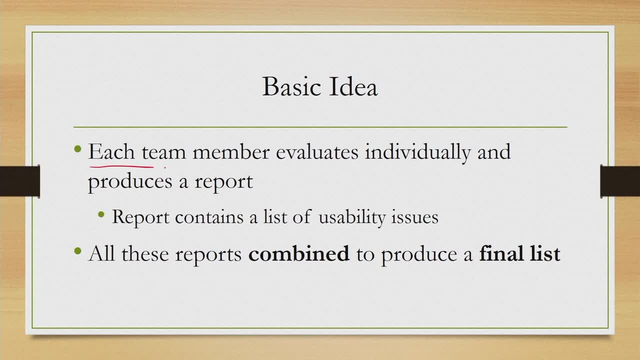 So what they do. So each team member evaluates individually and produces a report. Now, at the end of the evaluation, all these reports are combined to produce a final list What this list contains. Now, each report contains a list of usability issues and at the end, when we combine some 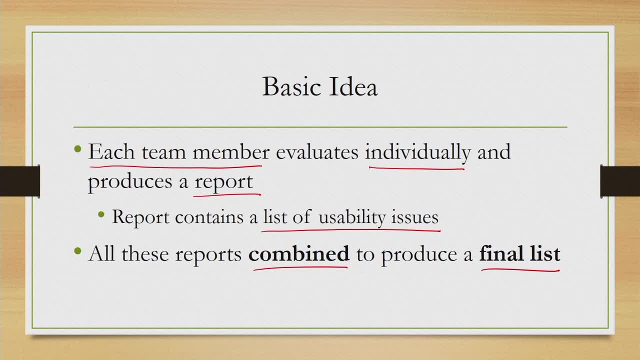 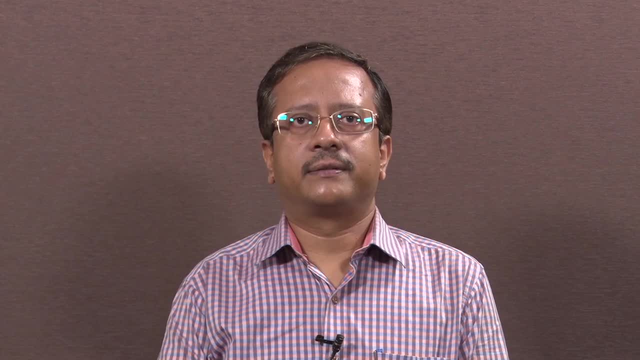 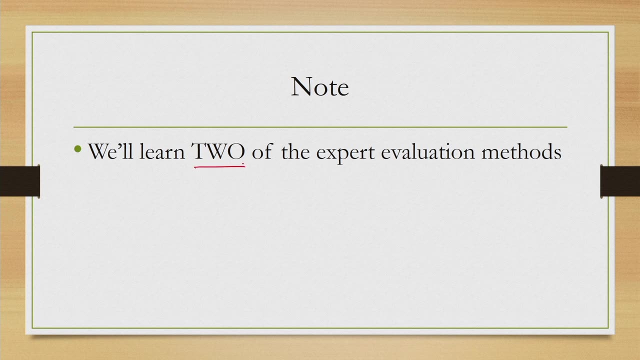 issues may be duplicated across the reports. those are removed and at the end it contains a list of unique, Unique usability issues identified by the evaluators. Now there are many expert evaluation techniques. we will learn two of those, namely the cognitive walk through and the heuristic evaluation. 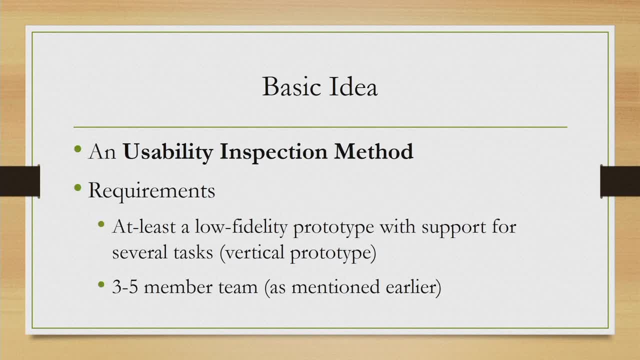 Let us start with cognitive walk through Now. this is an usability inspection method and its requirements are the same As that of any expert evaluation method. that is, we need at least a low fidelity prototype and a team consisting of 3 to 5 members, which may include- may include- the designers, some. 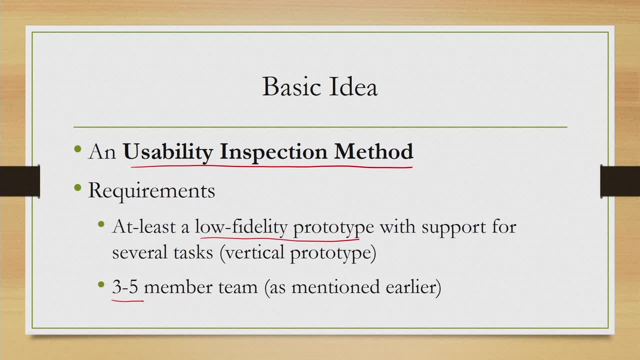 other skilled designers or end users. Now, in case of cognitive walk through, the prototype that we require should support several tasks, not a single task, And it should be developed as vertical prototype. Let us try to understand how to create this prototype and what we meant by support for. 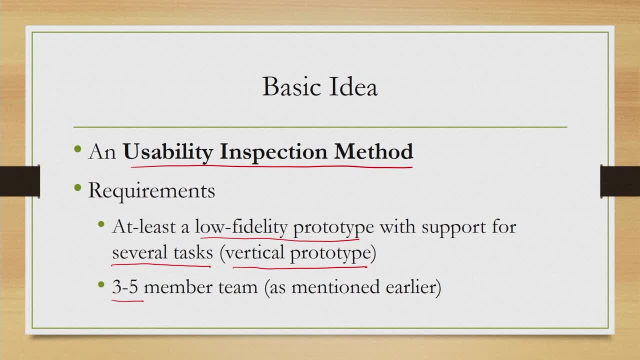 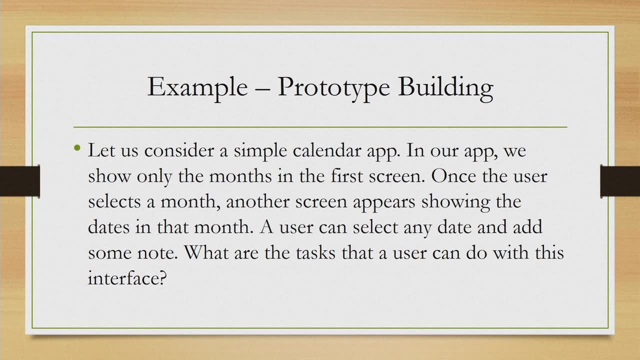 several tasks and vertical prototype in this context of cognitive walk through, Let us consider an example. Suppose we want to develop a simple calendar app. In our app we show only the months in the first screen and once the user selects a month, another screen appears showing the dates of the month. 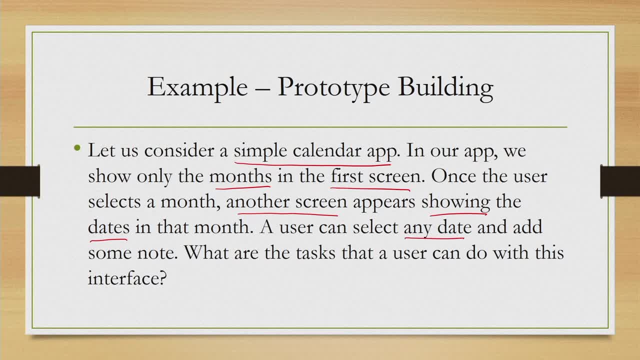 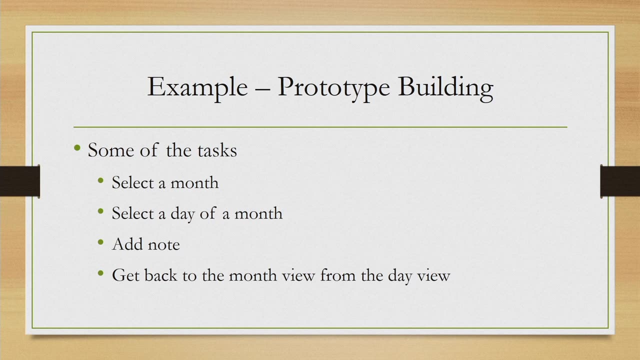 Now a user can select any date and add some note. So what are the tasks that a user can do with this interface? There can be several tasks. Let us see a few of those. One task can be select a month. another task can be select a day of a month. a third task. 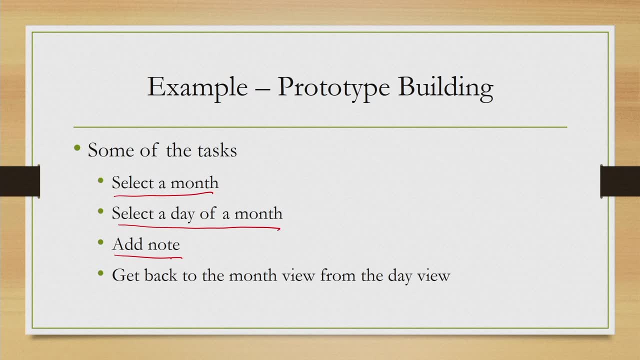 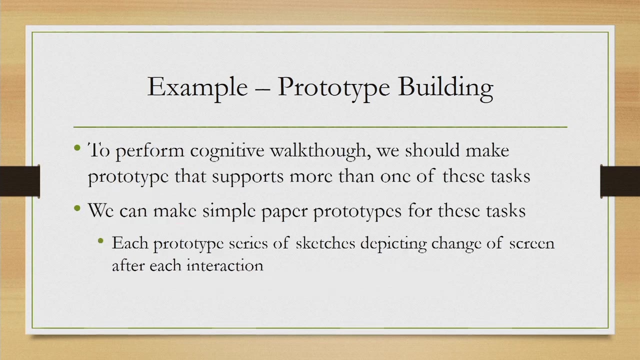 can be. add a note. fourth task can be get back to the month view from the day view. There may be other tasks as well Now, when we are talking of building a prototype for performing a cognitive walk through what we need to do. 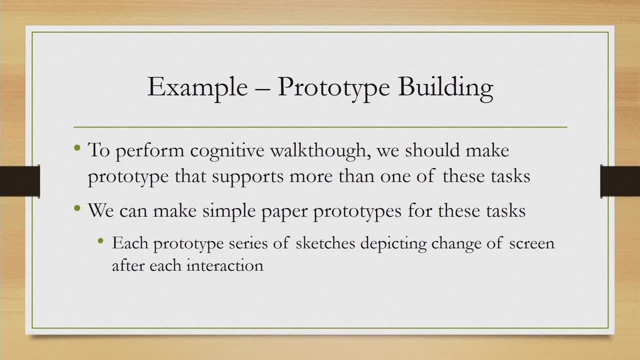 We need to build a prototype that supports more than one of these tasks. However, it is not necessary to go for very sophisticated prototypes. we can work with simple paper prototypes as well. that is why we called it low fidelity, And each prototype can simply be a series of sketches depicting the change of screen. 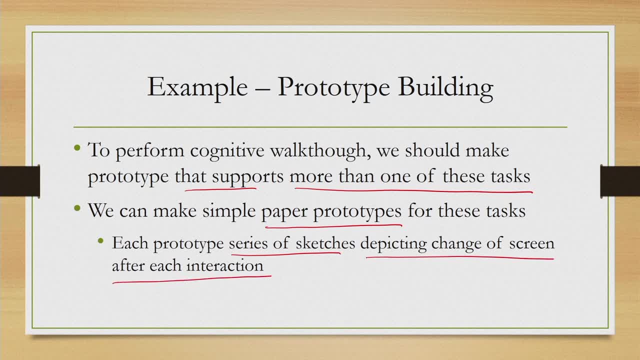 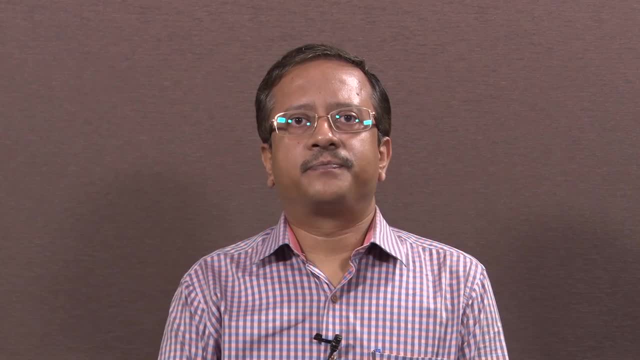 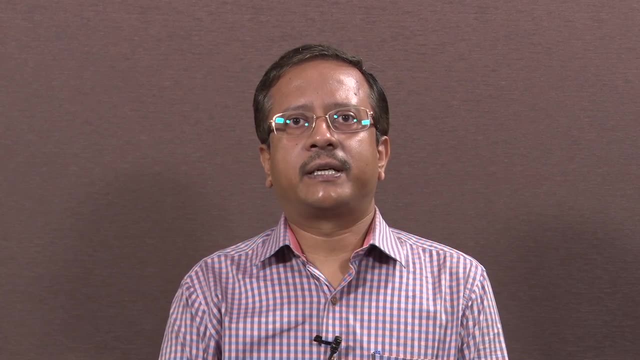 after each interaction. So when we say that we want to build a prototype to perform the task of selecting a month or a date, So for this task we can actually create a series of sketches depicting the change of screen when we perform the task. but since all the 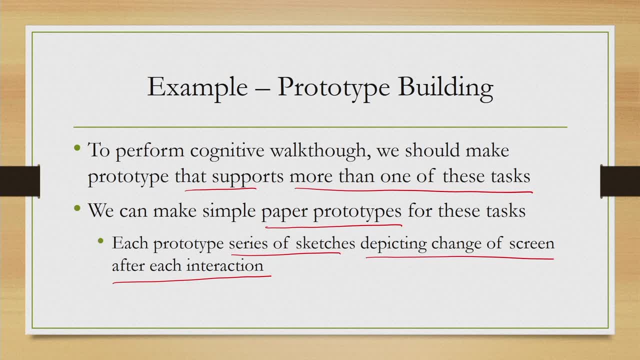 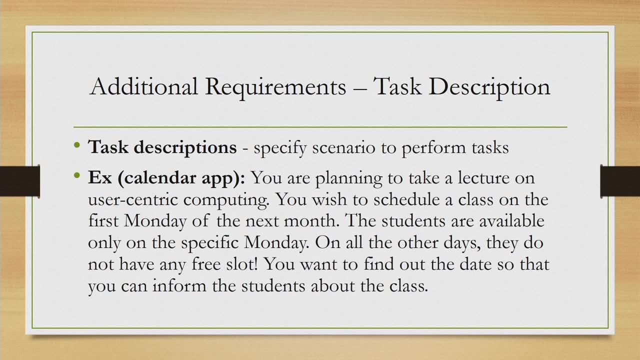 screens are depicted, So we are calling it a vertical prototype. So, along with those, that is requirement for a low fidelity vertical prototype for several tasks and design team. what else we require for performing a cognitive work through One is task description, as we have just seen before. what it means is specify the scenario to perform. 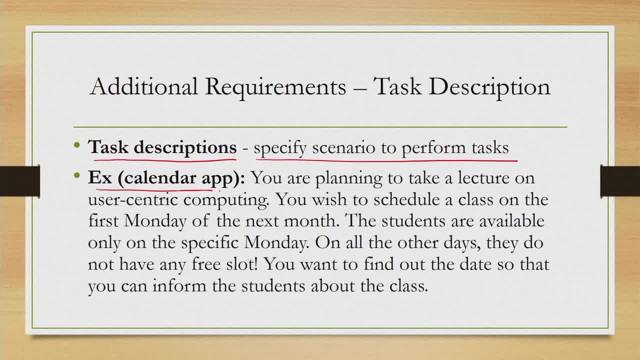 tasks. So for the calendar app example that we have just discussed, what can be a scenario, So one can be something like this: that you are planning to take a lecture on user centric computing. you wish to schedule a class on the first Monday of the next month. the students 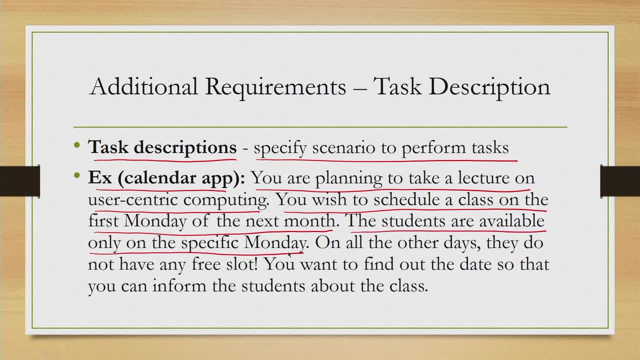 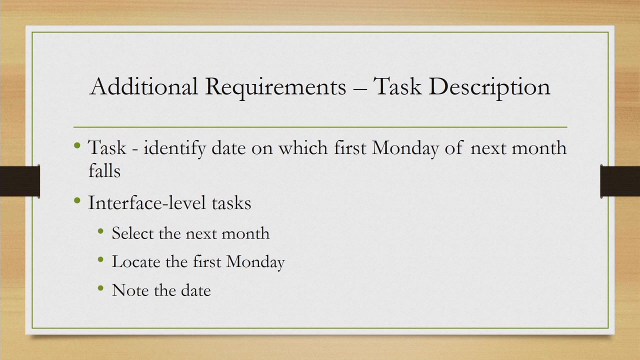 are available only on the specific Mondays. on all the other days they do not have any free slot. So you want to find out the date So that you can inform the students about the class. This is the usage scenario or task scenario. So, in order to achieve this, what we need to do We need to identify the date. 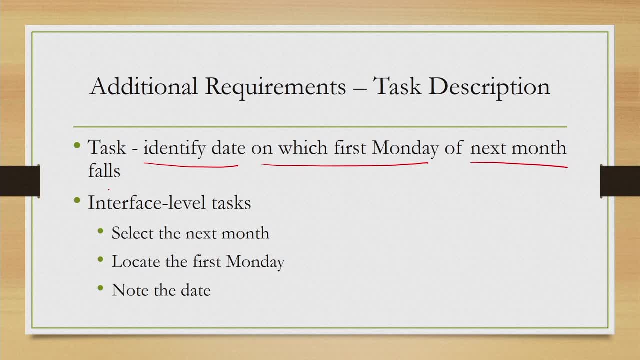 on which first Monday of the next month falls. So what are the sub tasks involved or the tasks that we need to perform on the interface involved in order to achieve this task? Select the next month, locate the first Monday and. 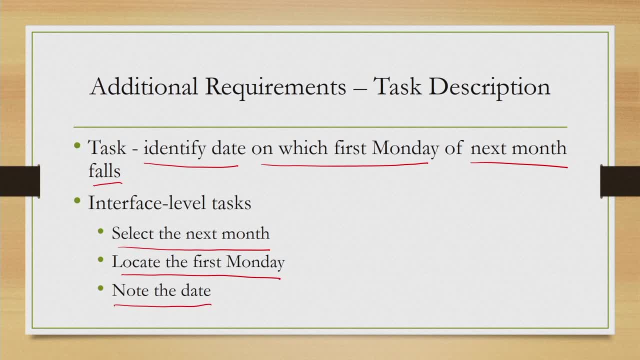 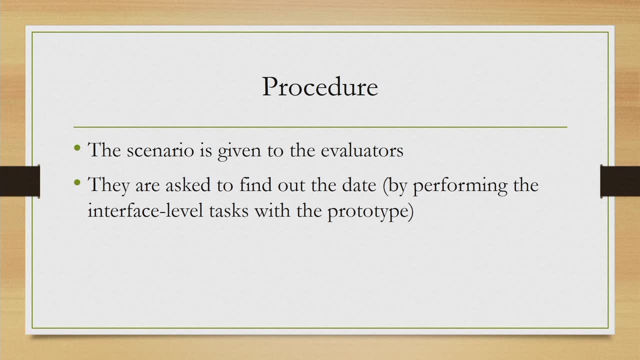 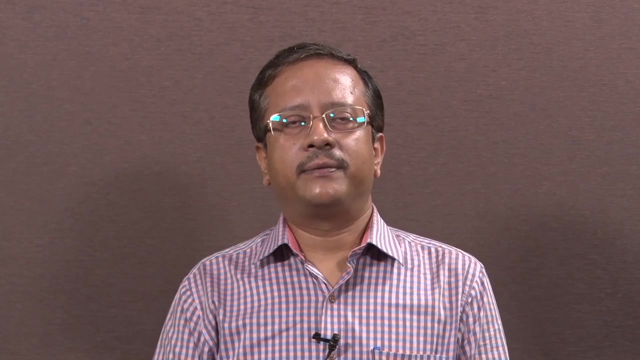 note the date. So if we can perform these tasks on the interface, then we will be able to achieve the overall task of identifying the particular date. So in cognitive work, through what we do. So we have selected all the next two dimensions taken from this statement. So this any out? 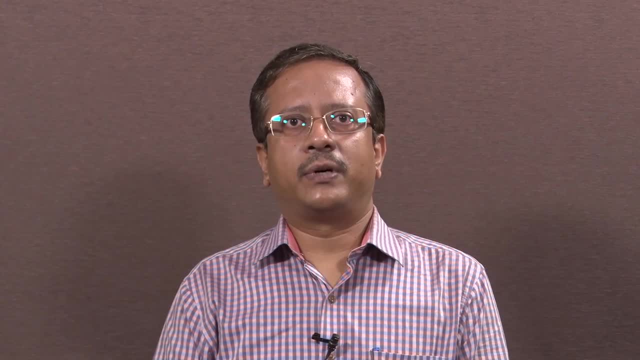 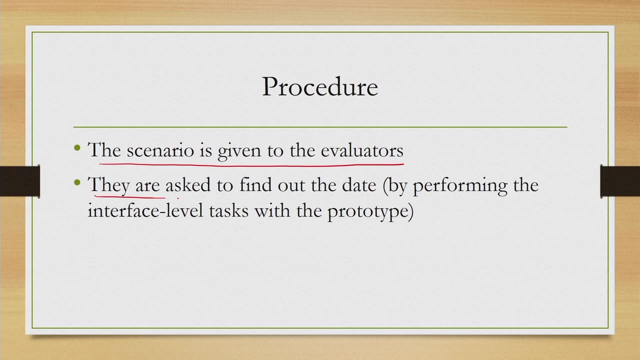 there we have 5 for 5 related tasks. Then it would be prepare with any packed information Next. so let us choose two tasks Here. I will not follow the смотреть task center just currently. 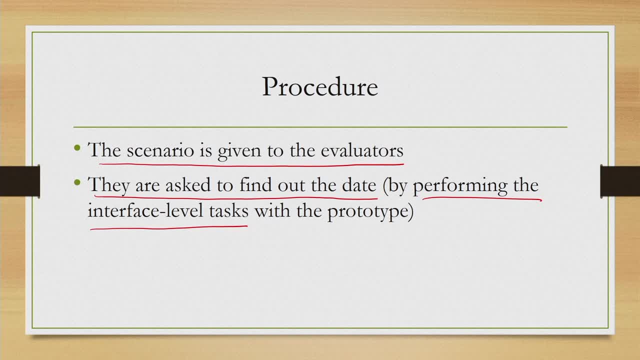 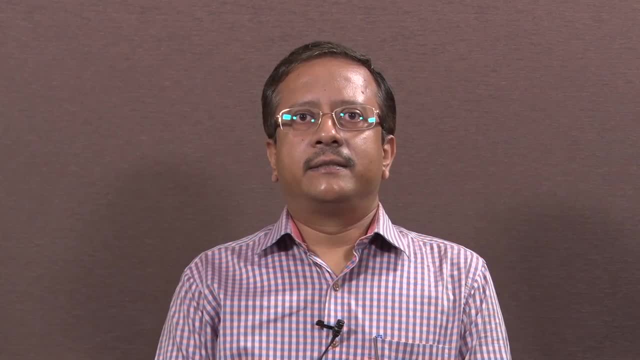 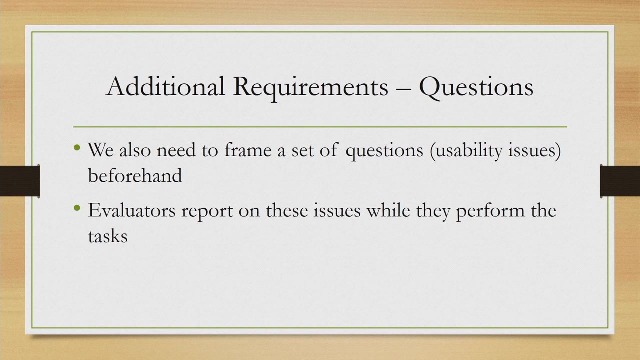 the interface level tasks with the prototype that is given to them, So each evaluator is asked to perform the task with the prototype. There is one more requirement: in order to perform a cognitive work through, We also need to frame a set of questions before, and so these questions are related to the 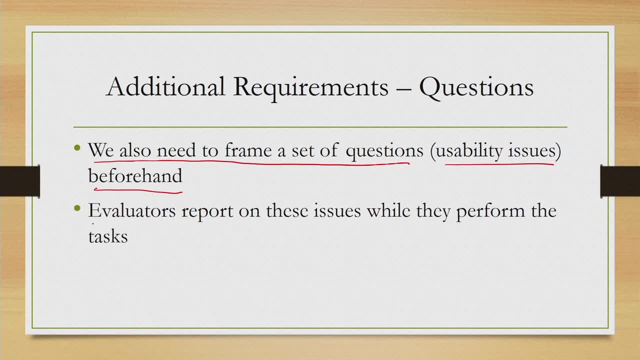 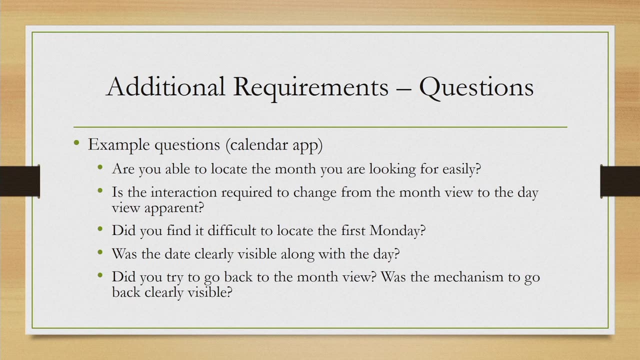 usability issues, and the evaluators are given these questions and they are asked to report on these issues while they perform the tasks. Let us see some example for our calendar app. What can be the questions? Are you able to locate the month you are looking for easily? 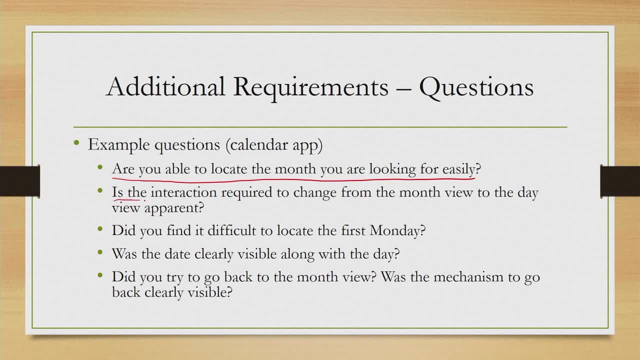 There can be another question, which is: is the interaction between the user and the user section required to change from the month view to the day view? apparent Third question can be: did you find it difficult to locate the first Monday? There can be a fourth question, which is: was the date clearly visible along with the day? 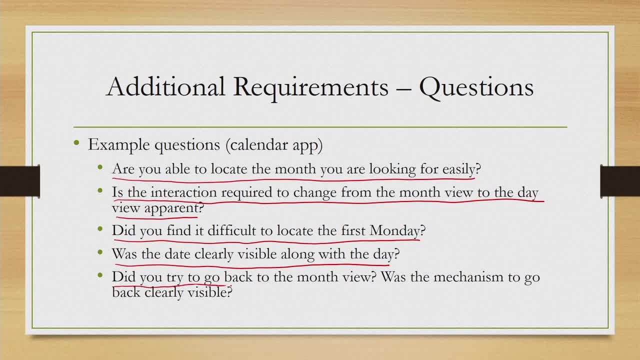 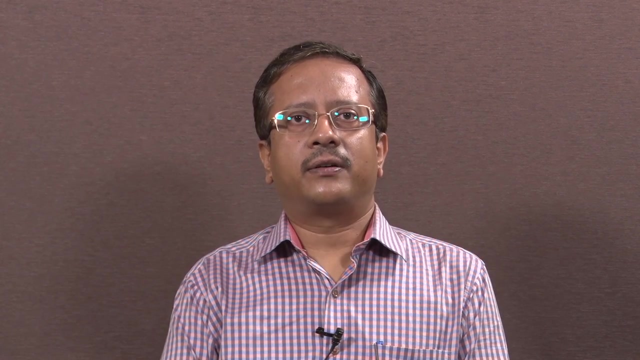 Even a fifth question. did you try to go back To the month view? was the mechanism to go back clearly visible? There can be many more questions. these are only some sample questions that can be given to the evaluators, So each evaluator will be given these questions and they will be asked to write their opinion. 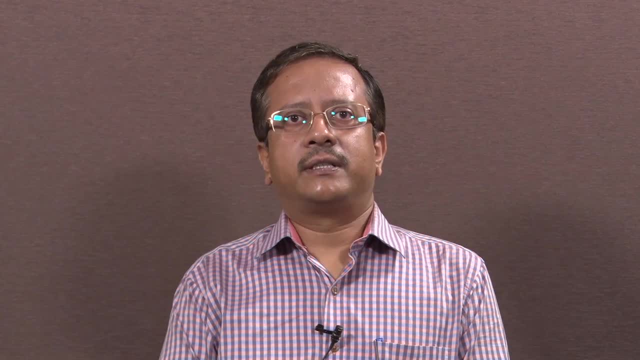 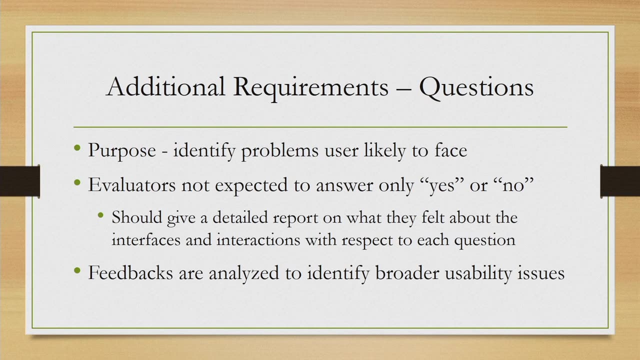 on each of these questions while they are performing the tasks with the prototype. What is the purpose of these questions? Purpose of these questions, as I mentioned before, to identify problems that the user is likely to face. So one very important thing is that the evaluator should not answer only in terms of yes or. 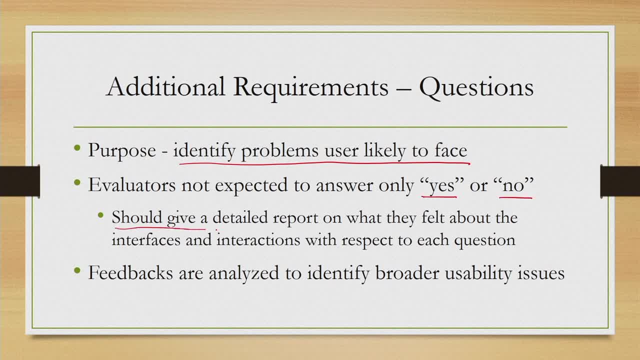 no. They must give a detailed report on what they felt about the interface and the interactions with respect to each question. So only a binary answer, yes or no, It will not be sufficient. Once the feedbacks are received from all the participants, from all the evaluators, they 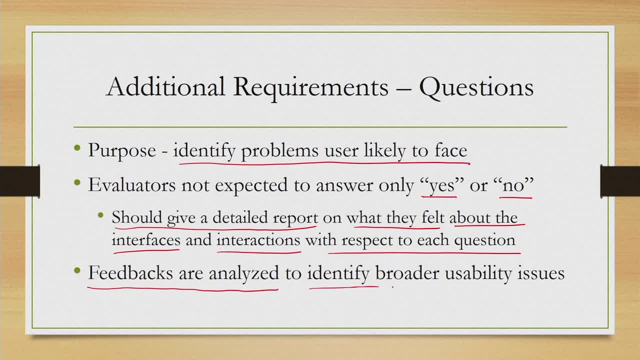 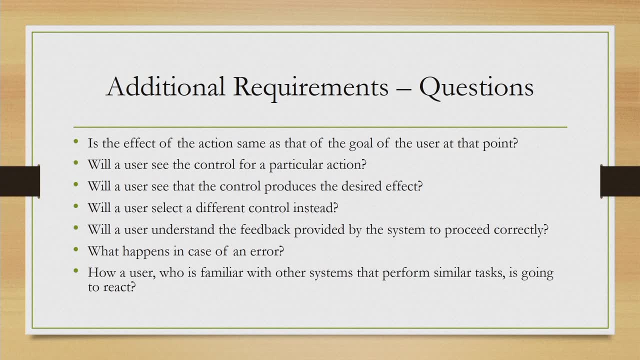 are compiled together and analyzed to identify broader usability issues. What are those broader issues? Few are shown here. As an analyst, you can try to answer these questions based on the feedback received. that is, Is the effect of the action same as that of the goal of the user at that point? 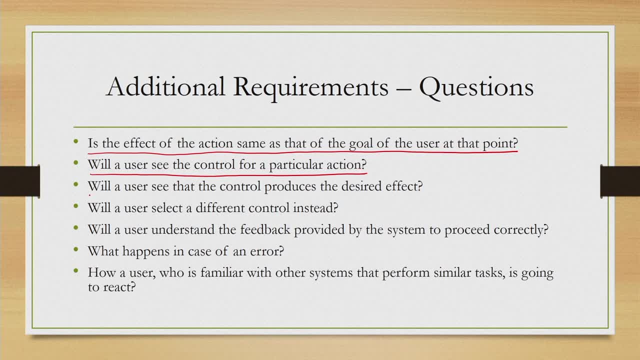 Will a user see the control for a particular action? Will a user see that the control produces the desired effect? Will a user select a different control instead? Will a user understand the feedback provided by the system to proceed correctly? What happens in case of an error? 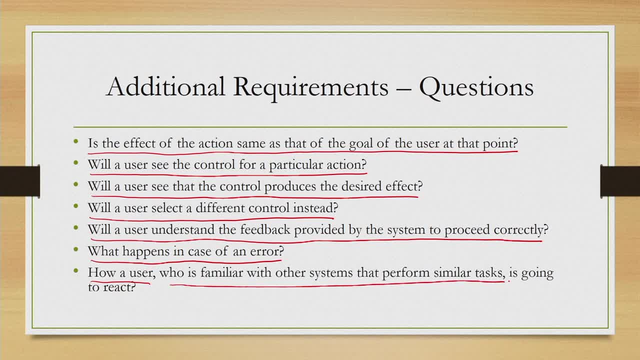 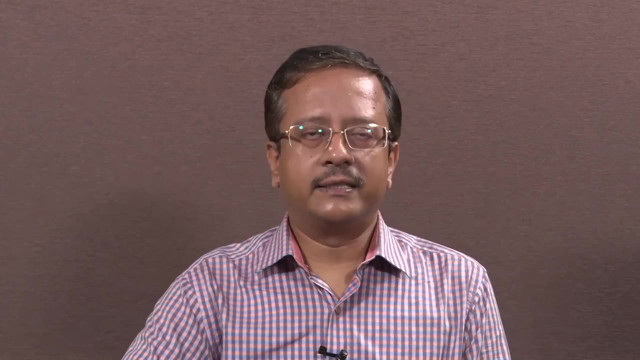 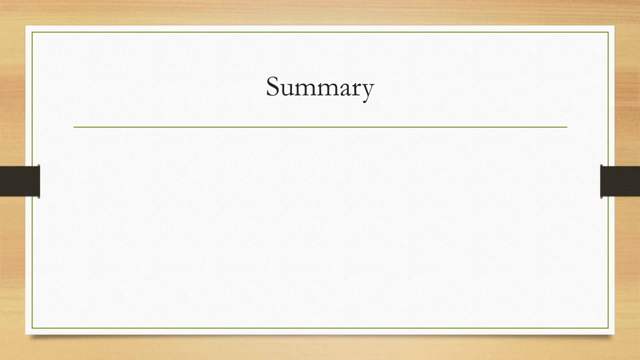 How a user who is familiar with other systems that perform similar tasks is going to react. These are some of the broader issues that can be answered based on the feedback received from the evaluators by analyzing their answers to each of the questions. So that is broadly what we are going to do. 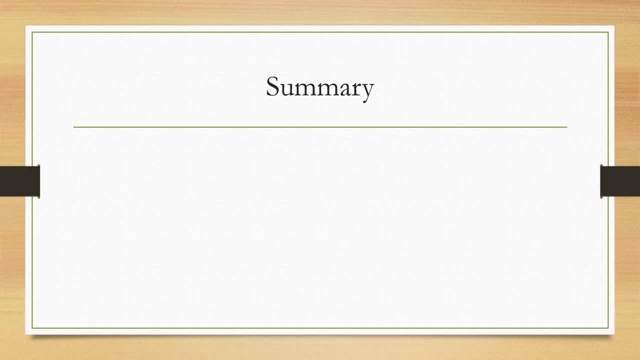 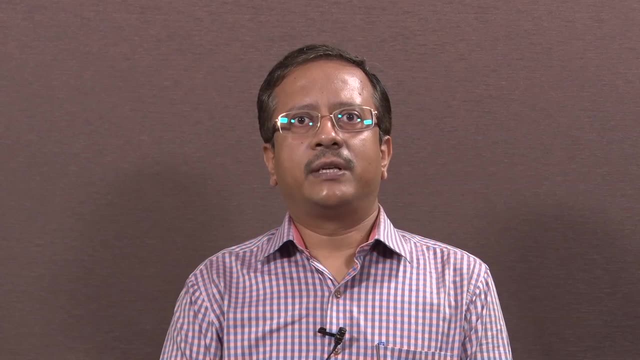 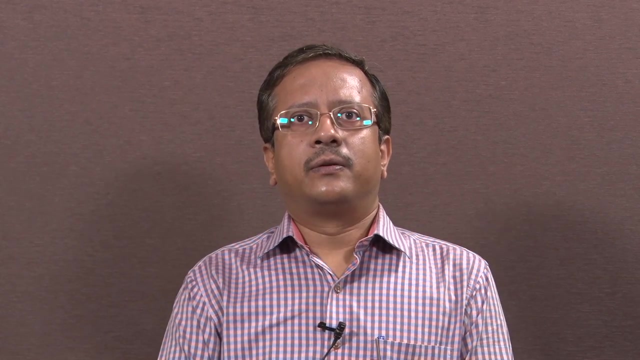 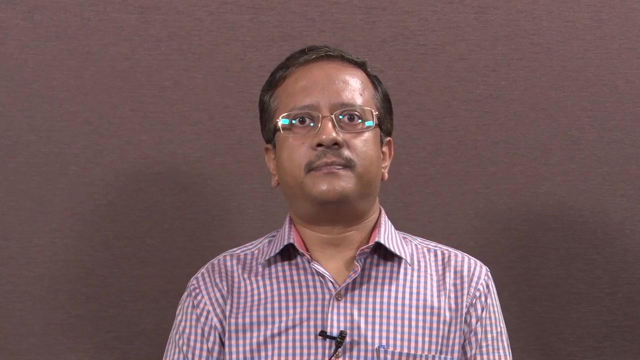 What we perform in a cognitive walkthrough, Just to recap. so we start with a low fidelity vertical prototype, for more than one scenarios preferably, and evaluation team comprising of 3 to 5 members. We frame the scenarios and, based on those scenarios, we create the prototypes. 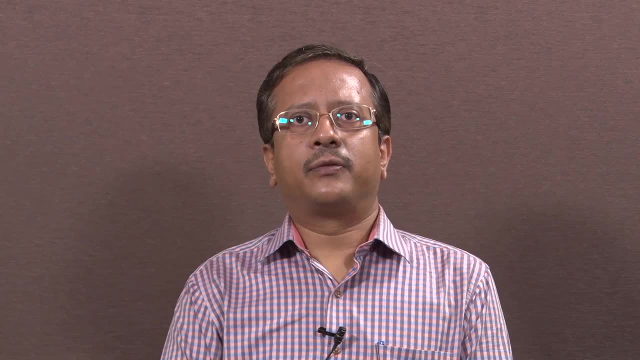 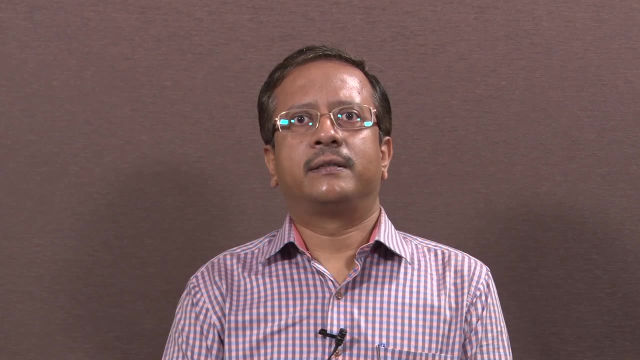 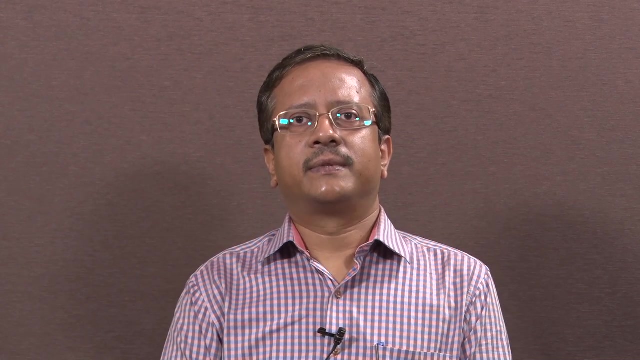 Each evaluation team member is given the prototypes Along with the evaluation team members. we create the prototypes. So we create the prototypes Along with the prototypes. they are given the task scenario and they are asked to perform the tasks. Along with that, they are given a set of questions and they are asked to give their opinion or 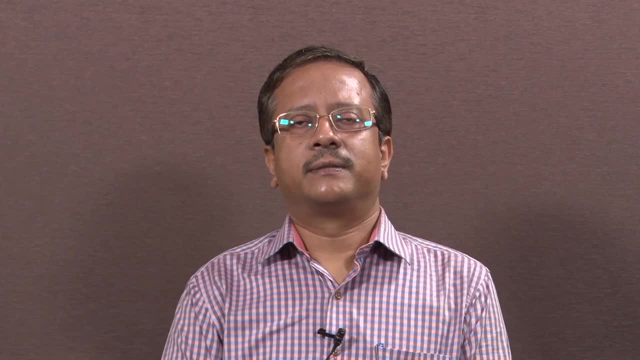 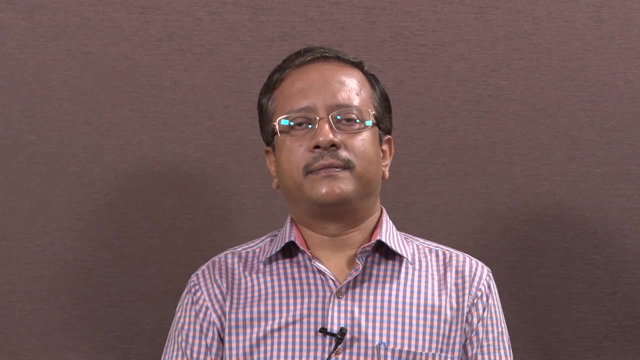 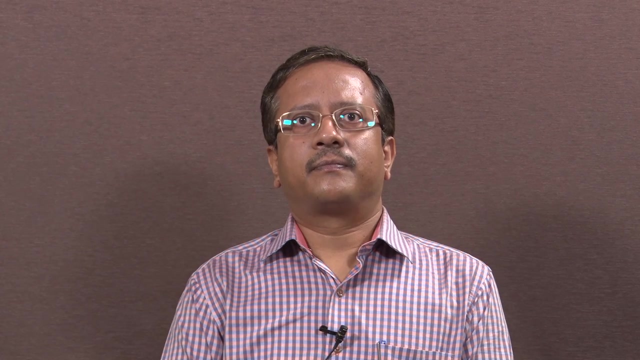 feedback for each of those questions while they perform the tasks. These questions are meant to elicit response on the performance of activity, So SUBSCRIBE AND FILL OUT, PLEASE. Thank you very much. Bye, bye of the interface and interaction with respect to a user and they are meant to identify broader 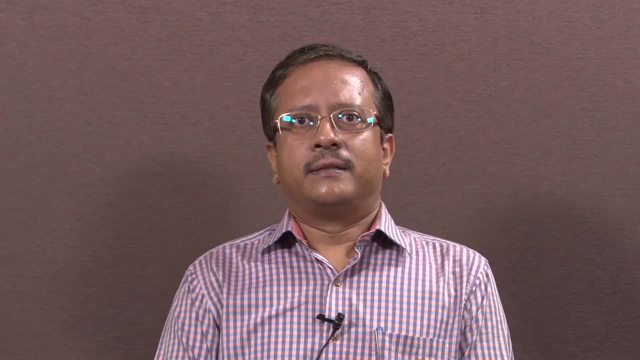 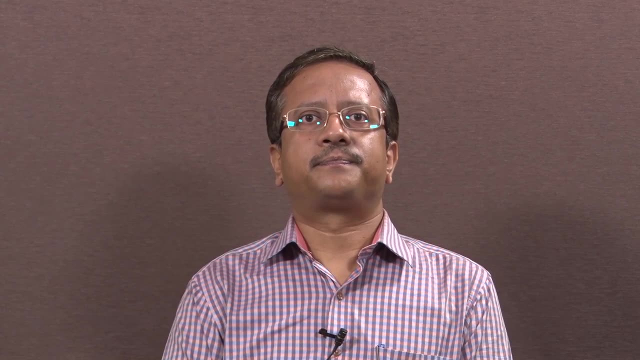 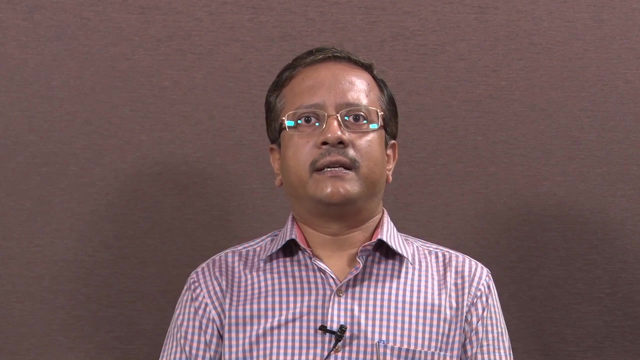 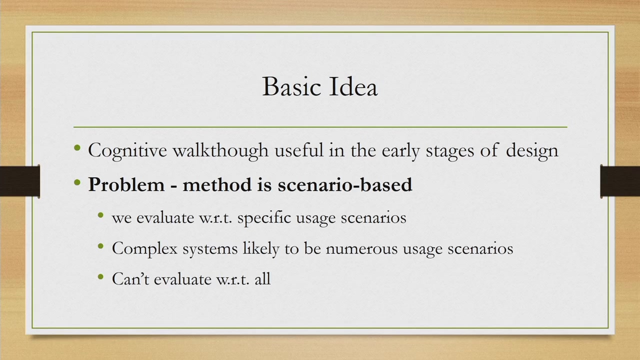 usability issues. So, as you can see here the issues are identified based on inspection of the interaction, inspection of the overall interface and interaction design. There is another evaluation technique which is called heuristic evaluation. In case of cognitive work through. it is useful in the early stages of the design. 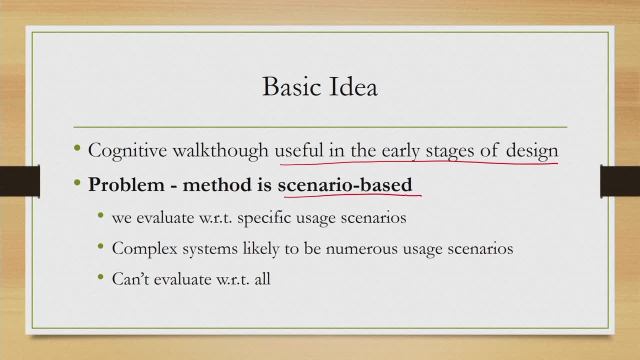 Now, the problem with this method is that it is scenario based, So we evaluate with respect to specific usage scenarios. So in case of complex systems, that is a problem, because complex systems are likely to have numerous scenarios and we cannot evaluate with respect to all. 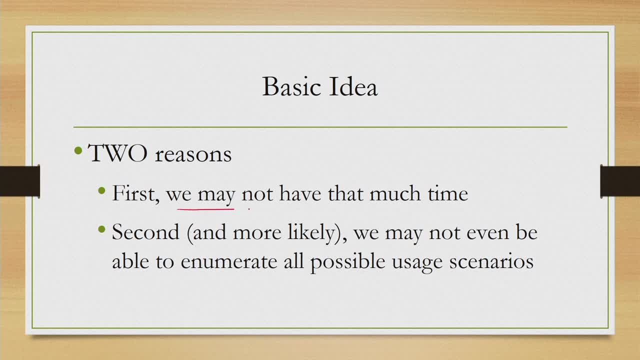 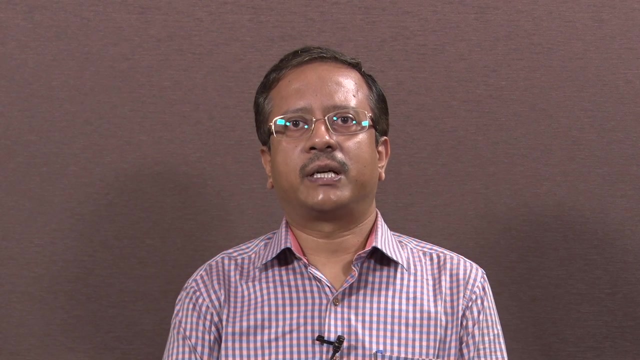 There are two reasons for that. first of all, we may not have sufficient time to do that. secondly, even if we have time, we actually may not be able to enumerate all possible usage scenarios. Okay, As an example, if you are using any advanced text editor to type messages such as Microsoft, 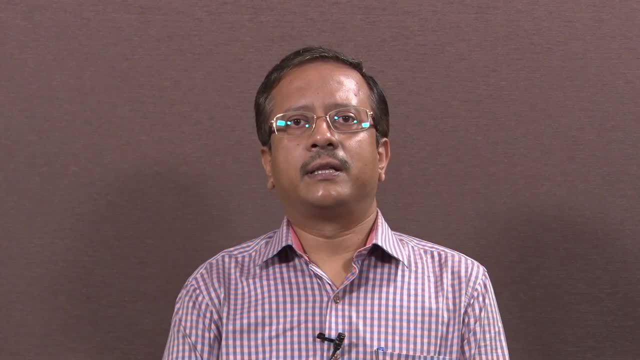 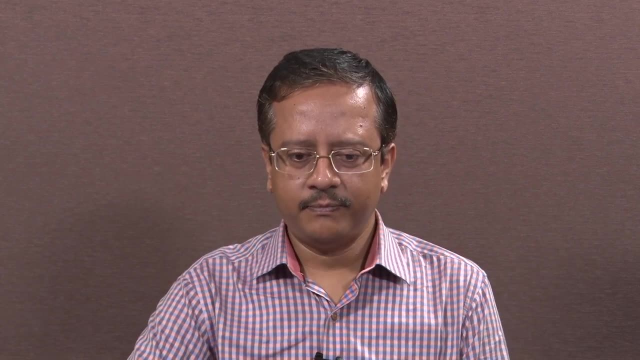 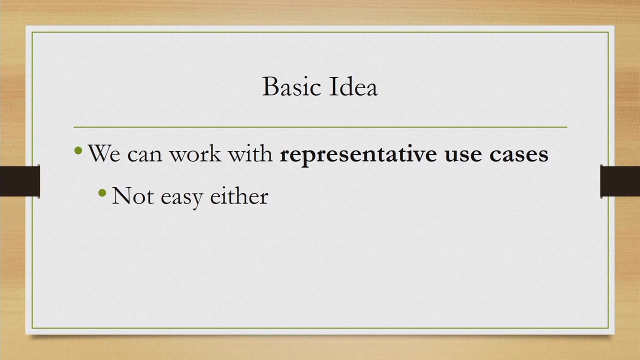 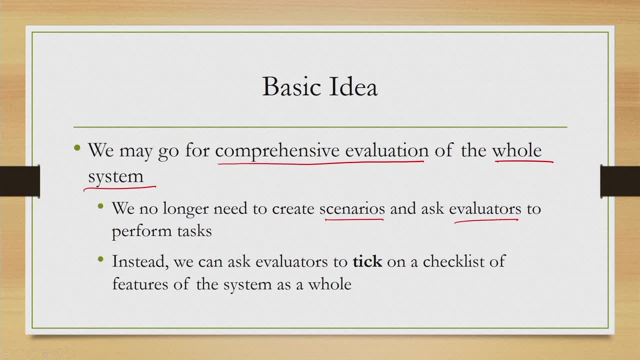 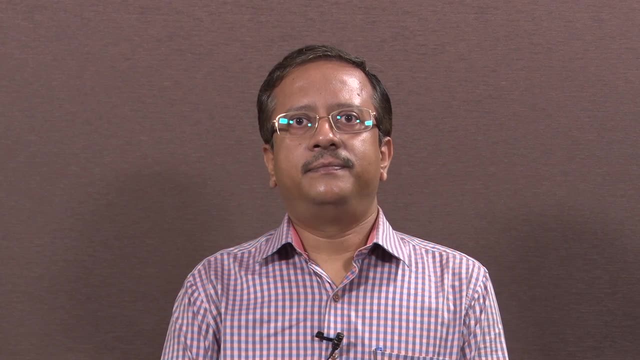 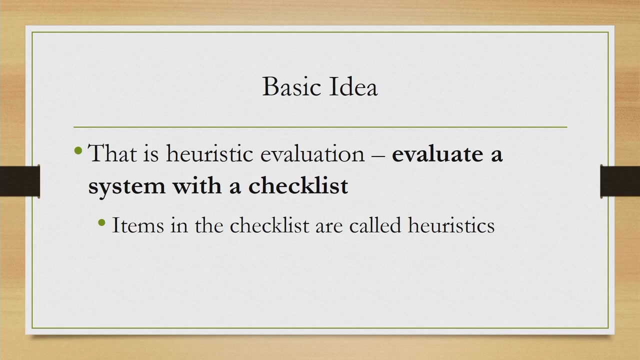 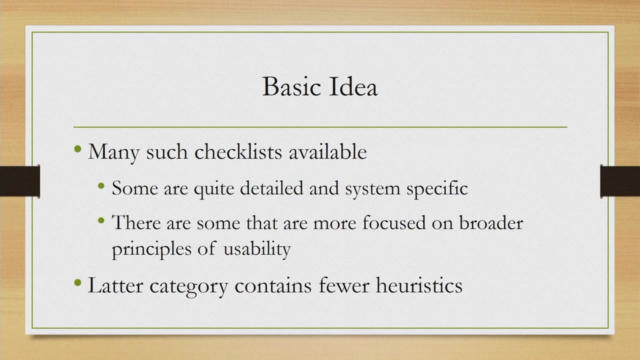 We evaluate a system with a checklist and the items in the checklist are called heuristics. There are many such checklists available. some are quite detailed and system specific and there are some that are more focused on broader principles of usability and clearly. 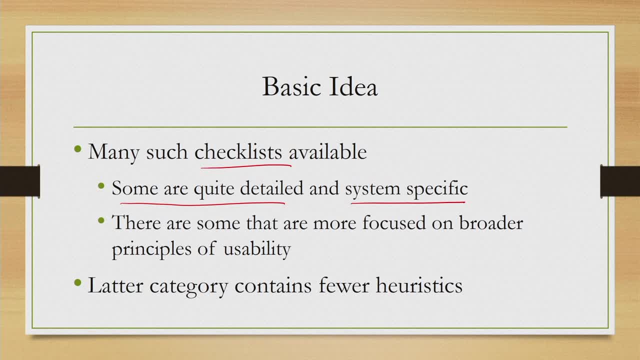 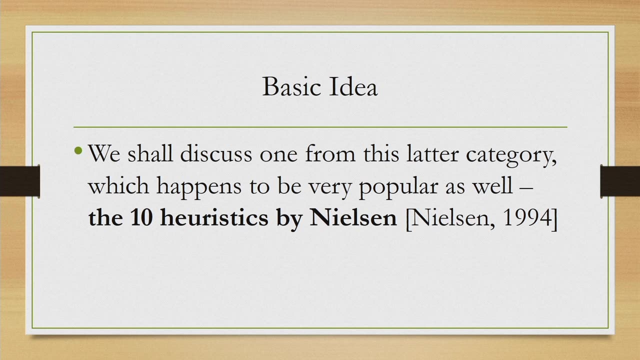 because of that reason, the corresponding checklists are having fewer heuristics. In this lecture we will discuss one from this later category of heuristics which focuses on broader issues, which is called the ten heuristics by Nielsen, or Nielsen's ten heuristics. 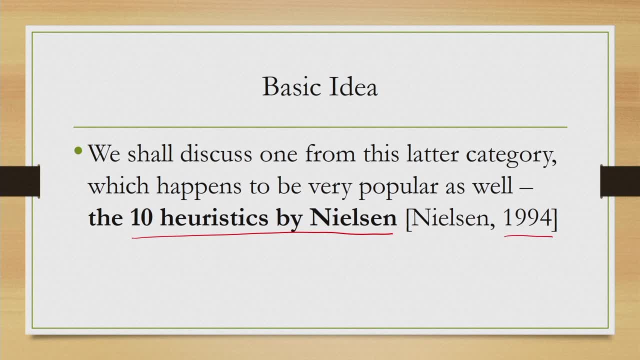 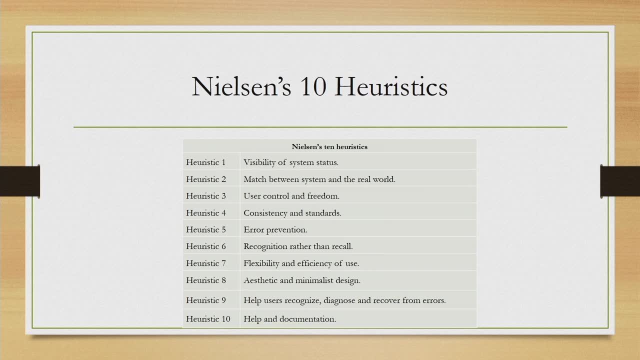 which was proposed by Nielsen in 1994.. Let us have a look at those ten heuristics as shown in this table. So heuristic one says the system status should always be visible to the user. What it means is that the users should always get a feeling of what is going on in the system. 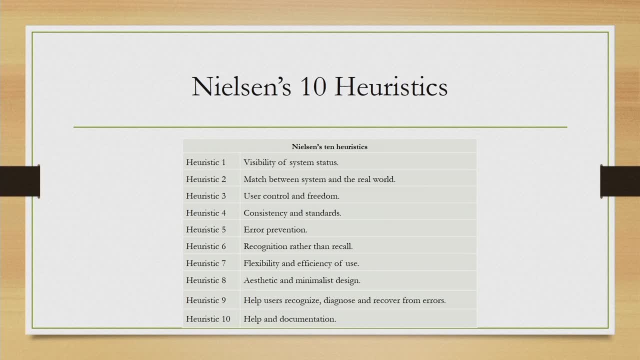 So essentially it refers to some sort of feedback for system activities which should be given to the user for whatever tasks he or she performs. Not only that, it also tells that the feedback should be given within a reasonable time. It should not be too late so that it is difficult to relate the feedback with the activity. 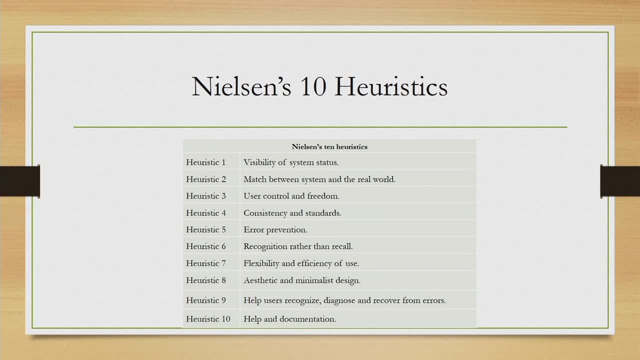 A time is mentioned which is 500 milliseconds. So essentially what it tells is that give feedback within 500 milliseconds, then it will be more effective. In heuristic, two tells is that there should be a match between the system and the real world. So whatever. 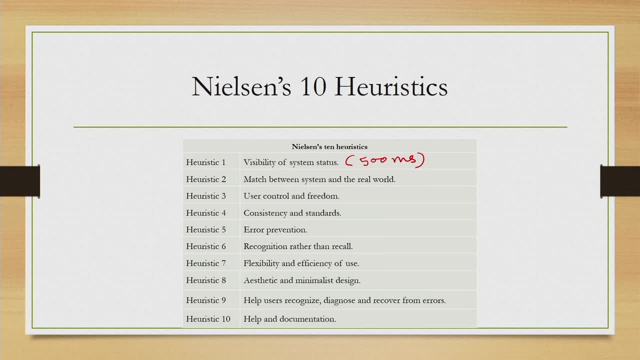 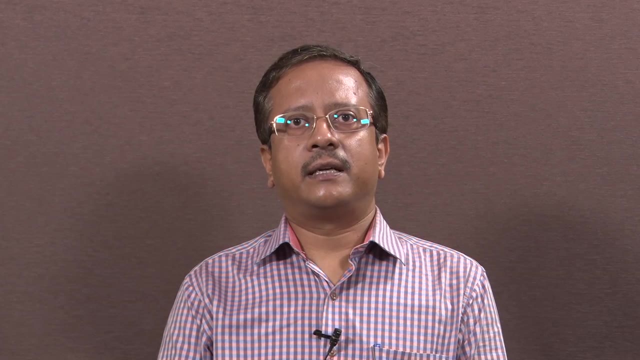 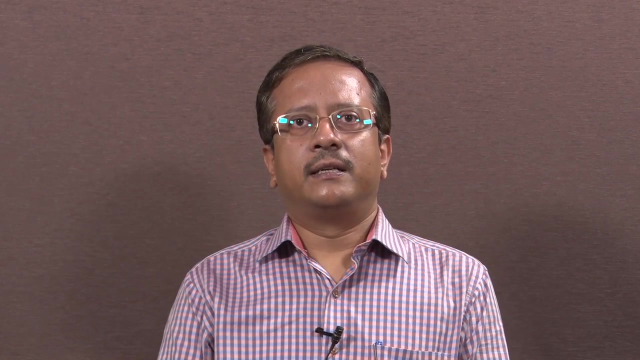 we get to see in the real world should be used, to the extent possible, to design things in the system So that there is some consistency between our experience in the real world and or experience in the virtual world. If you may recollect, earlier we talked of guidelines. 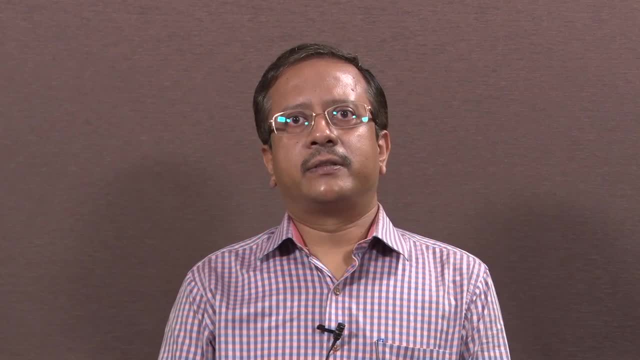 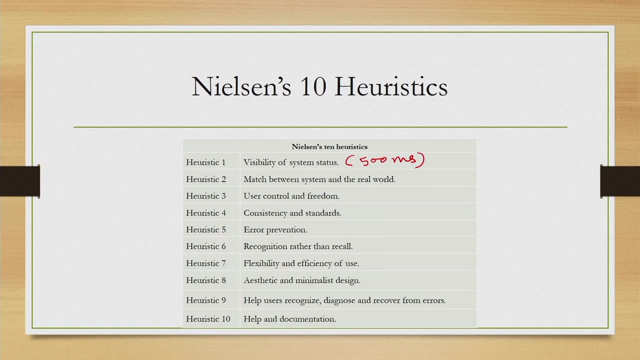 there we talked of external consistency, consistency between the system and the real world. This heuristic essentially points to the same. the third is user control and freedom. So this third is user control and freedom. So this third is user control and freedom. this third is user control and freedom. So 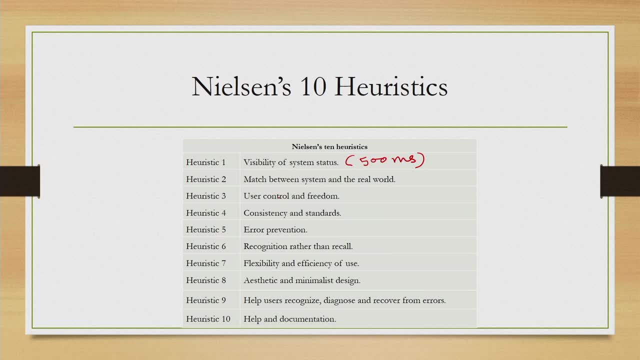 Third heuristic refers to the refers to the fact that the design should have undo and redo facilities, because users may make mistakes and they should be able to come out of those mistakes without going through elaborate dialogues. So if they can come out quickly, then they feel that they are in control and they have 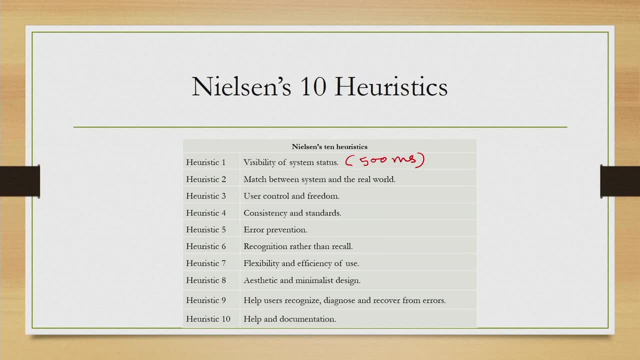 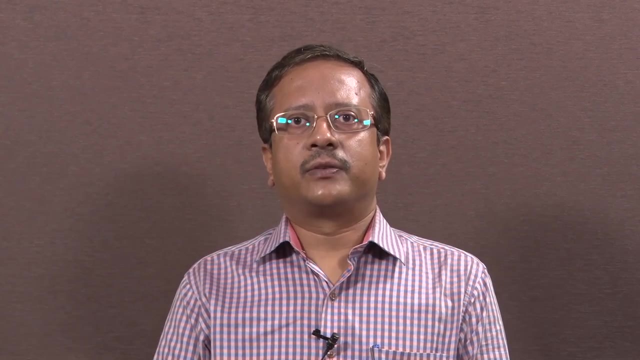 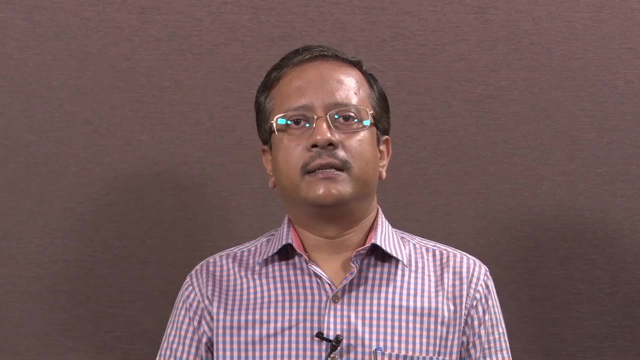 freedom to do whatever they wish. Point 4 is on consistency and standards. that is, throughout the system. you should follow some consistency and it should follow standards so that every time the user need not learn new things. essentially, it refers to internal consistency in the system. 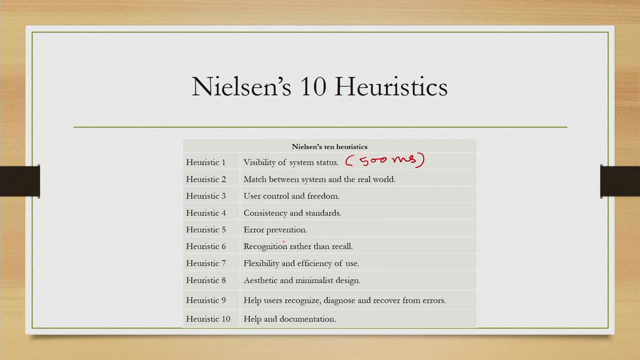 The concern of designs that helps the user to prevent errors. So this is taken care of in heuristic 5, that we should go for designs that prevents occurrence of errors. Heuristic 6 is interesting. what it tells is that whatever you do to design the system, 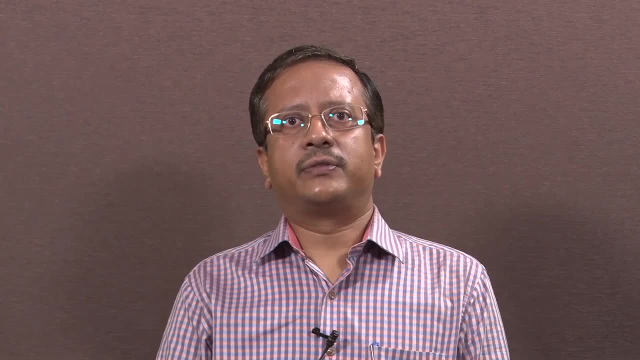 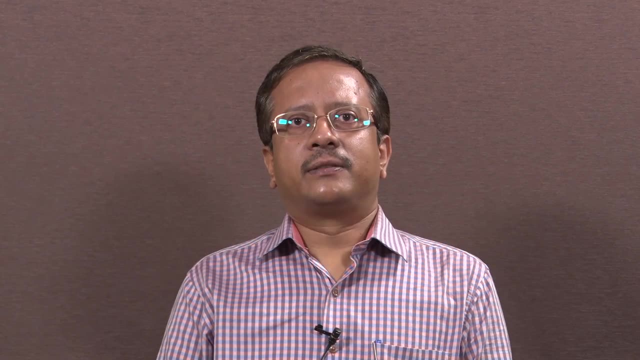 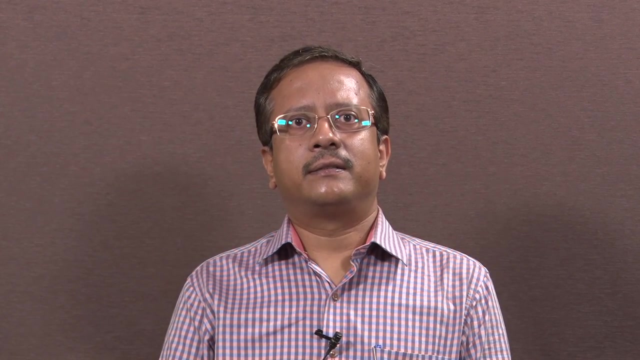 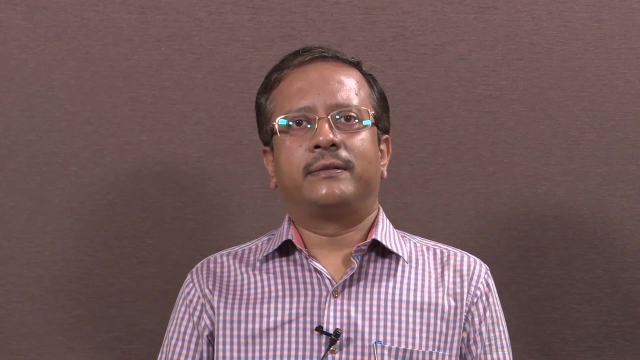 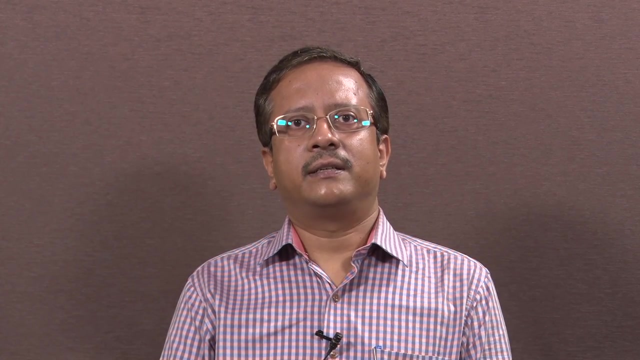 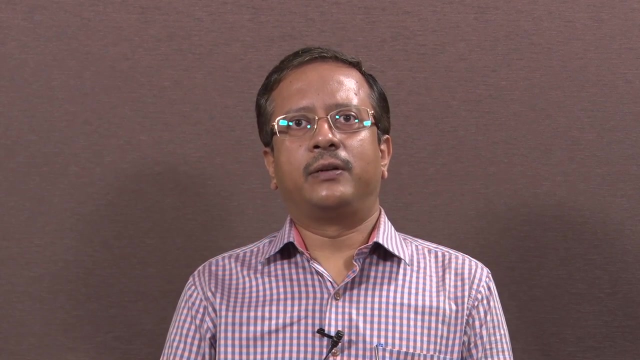 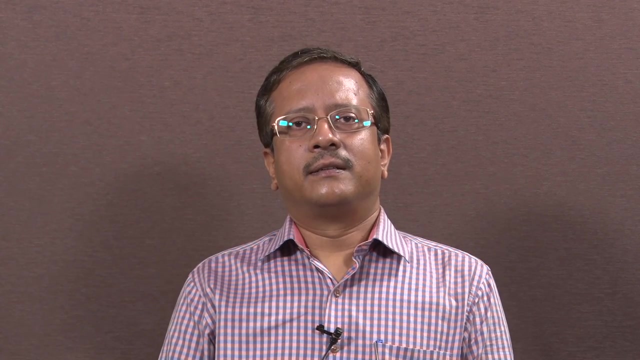 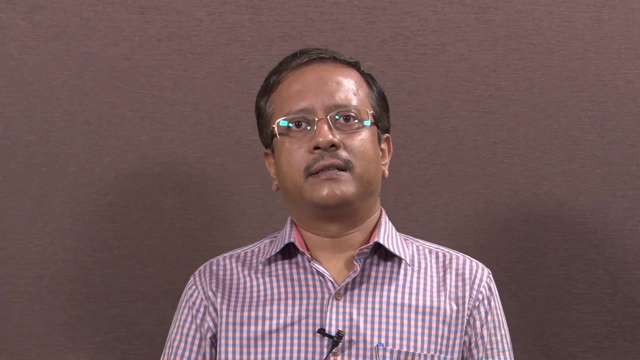 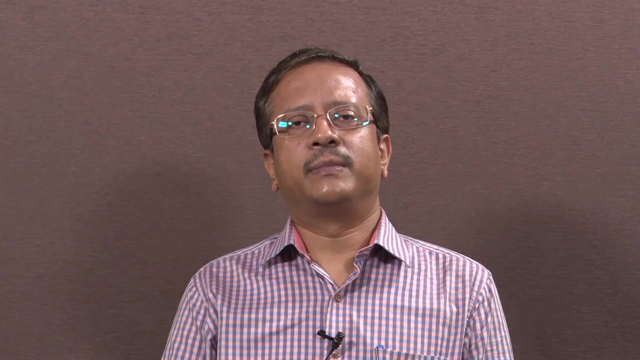 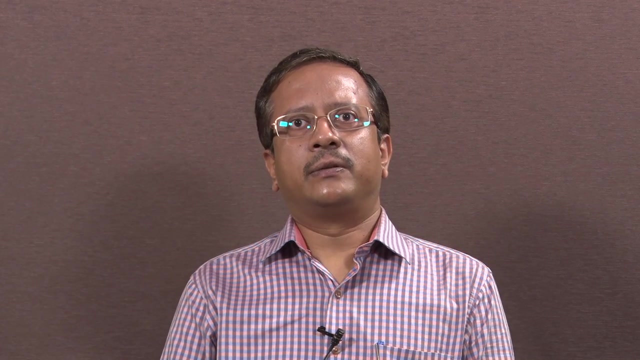 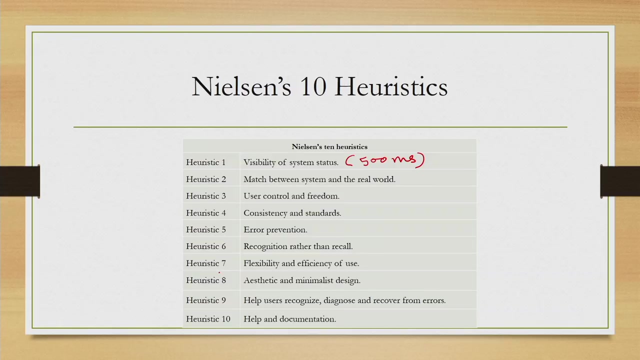 should help the user recognize the purpose rather than forcing the user to recollect the purpose. So what is the use? essentially, it refers to the fact that whenever you design, we should keep in mind different categories of users, namely the expert users, novice users, intermittent. 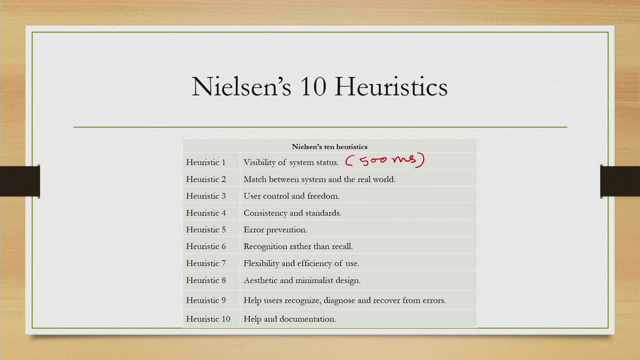 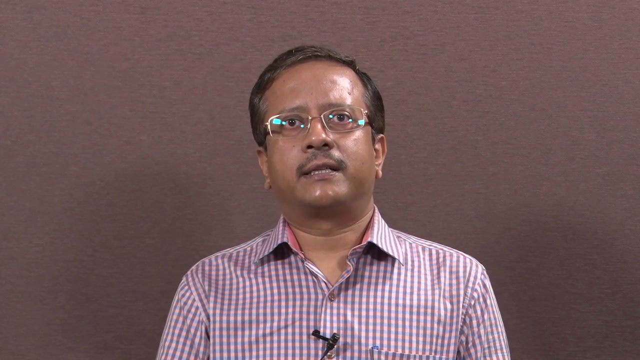 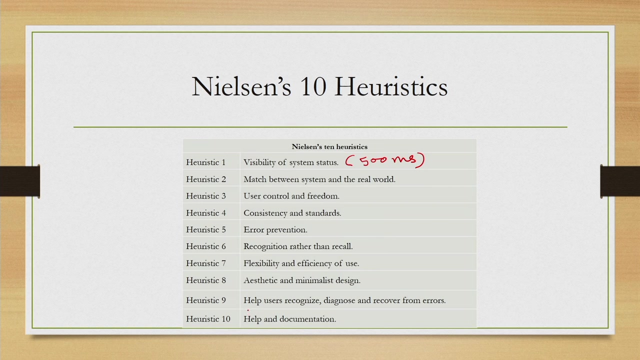 users In the eighth heuristic. the eighth heuristic refers to a simple design which looks aesthetically pleasing and minimalist, that is, it avoids redundancy. It is expected that such designs help in satisfying the users. In the ninth heuristic the fact that human makes mistakes, irrespective of how well the 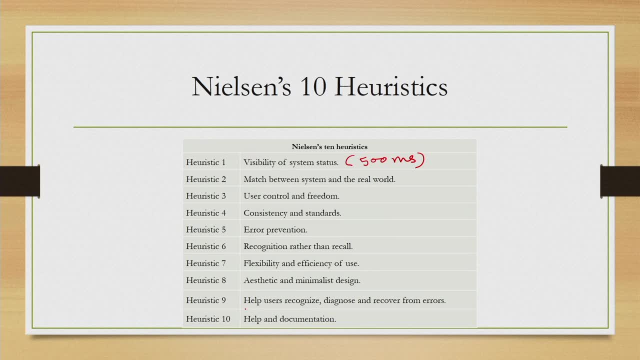 design is has been taken care of. It says that help users recognize, diagnose and recover from errors, So it assumes that there will be errors irrespective of how well the design is. but the design should support the user to recognize, diagnose and recover from errors. 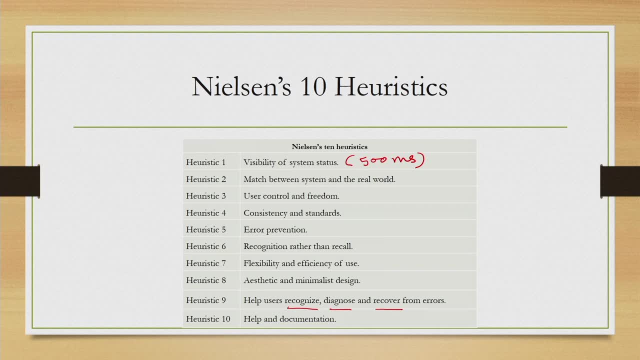 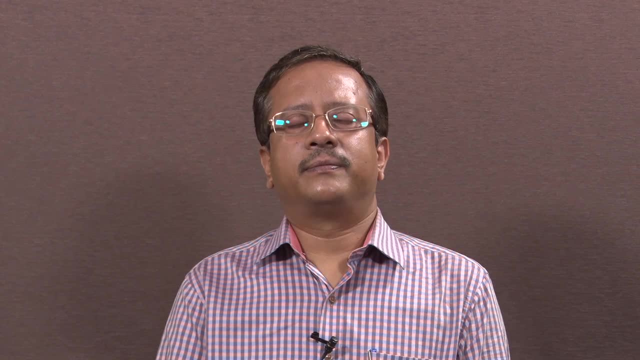 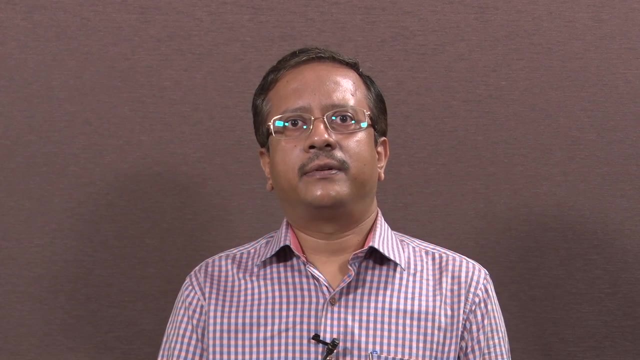 So we should not give some very cryptic error messages to indicate the occurrence of an error. Instead, it should produce some errors, So understandable messages, preferably in natural language, and produce some friendly advice on how to recover from the error and what are the likely consequences. 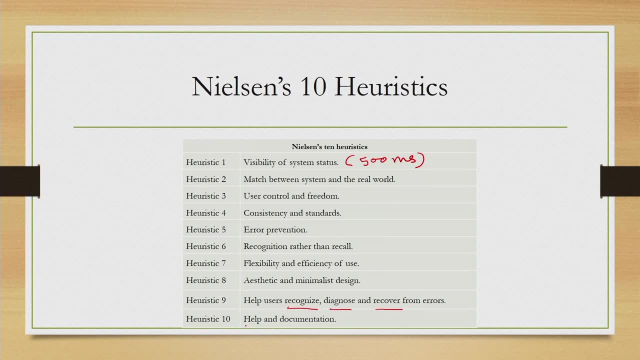 Finally, in heuristic 10,, it is emphasized that any design or any system should have suitably designed help and documentation, where the object should be easily identifiable and searchable. Together, the set of 10 heuristics has been designed to ensure that usability concerns. 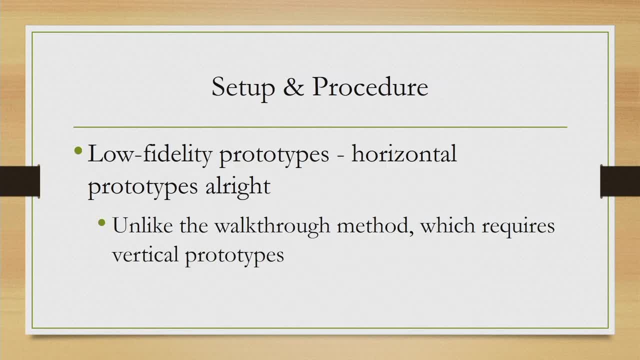 are taken care of in a design. So in order to perform heuristic evaluation- what we do Again- we require a low fidelity prototype, but in this case we do not require vertical prototypes. Vertical prototype is fine. This is in contrast to the walkthrough method, where we require a vertical prototype. 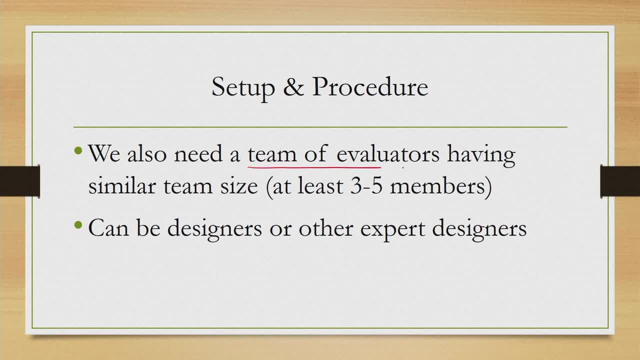 The second requirement is same, that is, we require a team of evaluators having at least 3 to 5 members, and this team can have designers, can have other skilled designers or may also include 1 or 2.. So this is a very simple evaluation process that I have given to users. 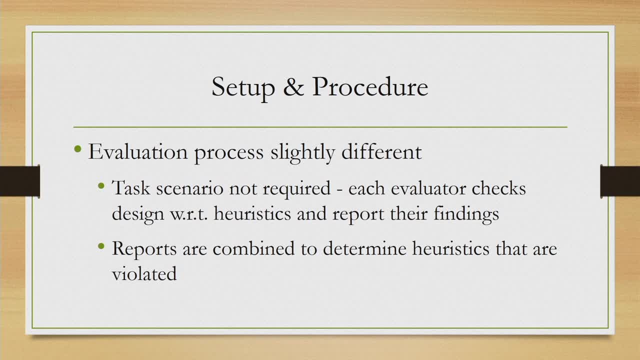 The evaluation process, however, is slightly different. Earlier, we asked the users to perform the tasks specified in the scenario. Here we do not do that because we do not have any task scenario. So what we tell each evaluator is to check the design with respect to the heuristics.